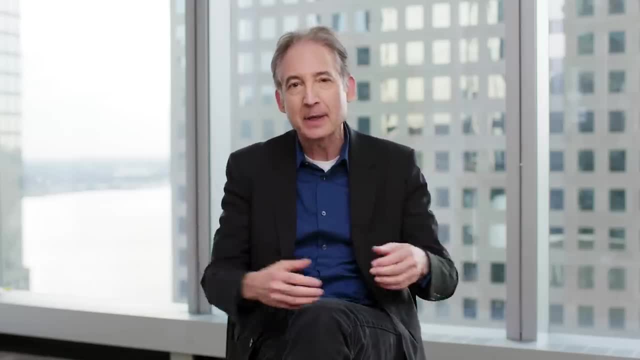 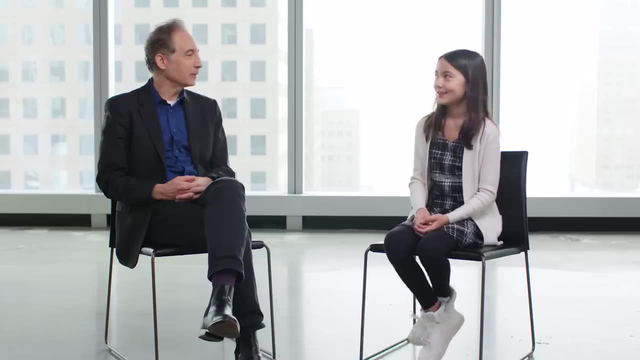 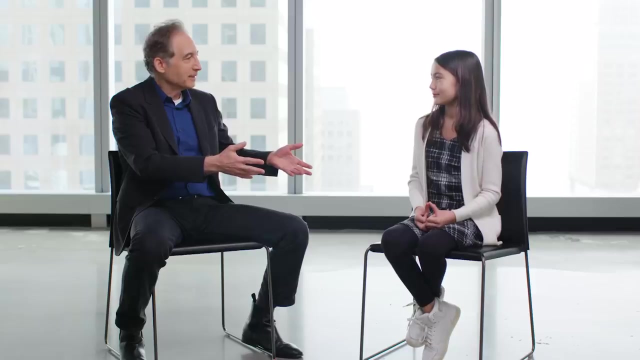 some duration of time. so if you can understand time, you're on your way to understanding reality. Hello, Hello, What's your name, Kayla? How old are you, Kayla? I am nine years old. So if you're nine years old, what does that mean about the earth? How many times has it gone around the sun? 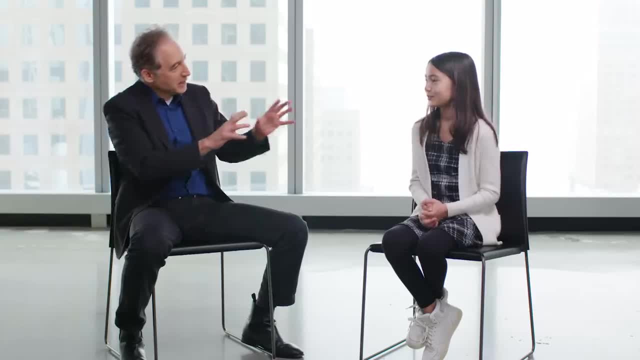 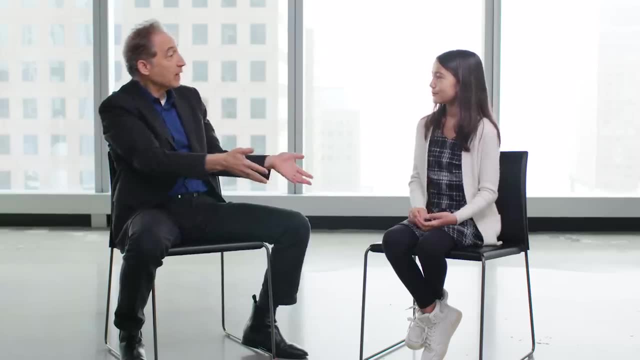 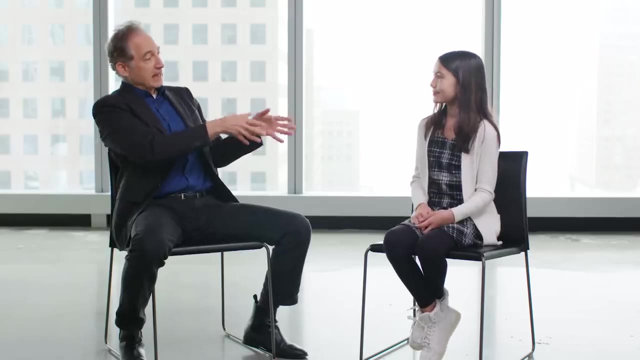 Nine times Nine times. So there's a relationship between motion through space- the earth is going through space- and the passage of time. They're kind of connected in some way, But there are differences. right? If I asked you to move through space, 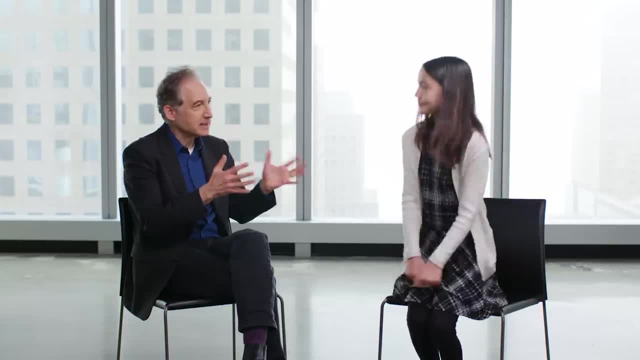 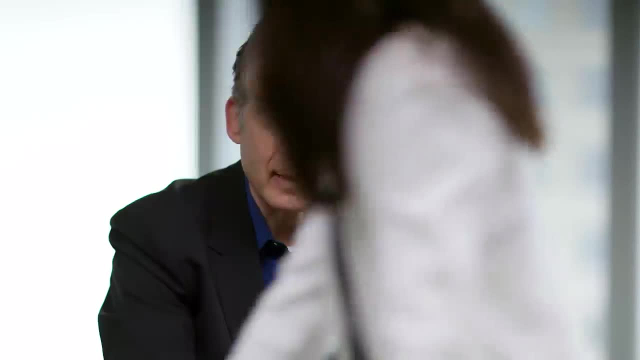 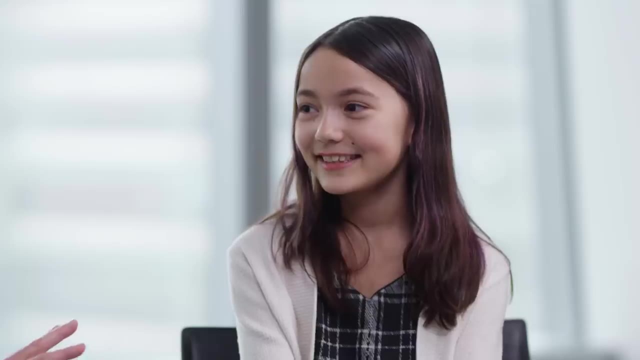 you could do it freely, right? Can you get up And let's see how easy it is to move through space? Can you move over to that location And can you come back? Anything getting in your way Easy to do? Yep, If I were to ask you to sit perfectly still in space, can you do that? I mean hold. 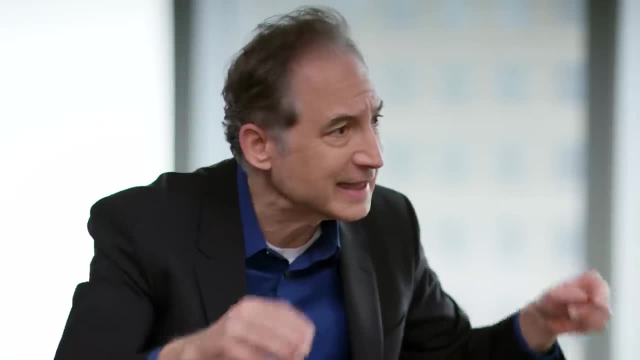 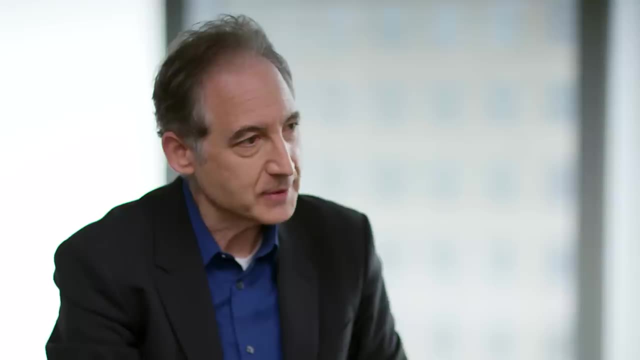 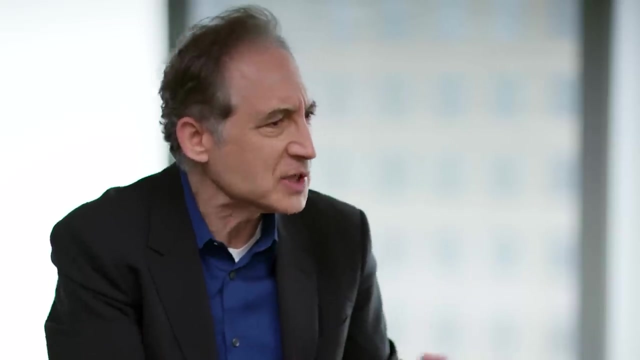 perfectly still. That's good, But if I ask you to hold still in time, to not go to the next second or the next second, can you do that? No, So there's definitely. there's definitely. there's definitely this difference between space and time, some fundamental quality that distinguishes how freely 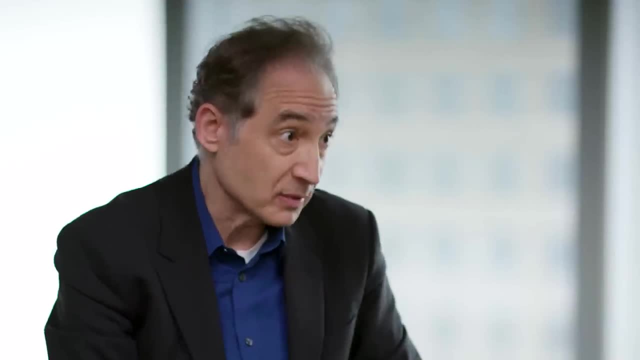 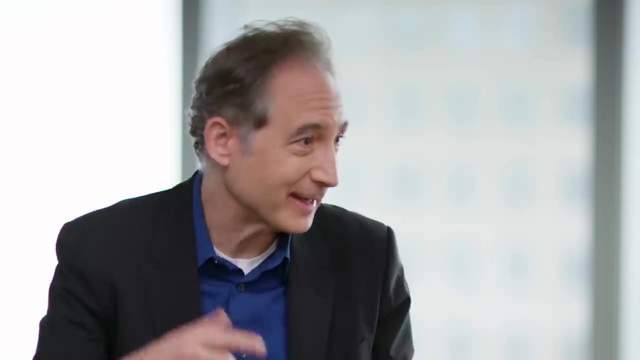 we can move through space versus how freely we can move through time. Have you heard of Albert Einstein? Yes, What do you know about him? He has crazy hair. He does have crazy hair, and I think I may be heading in that direction, actually. 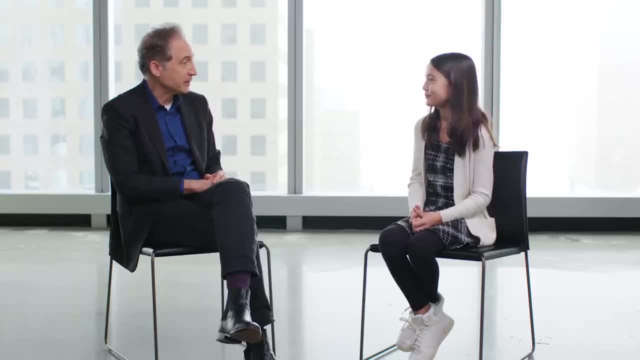 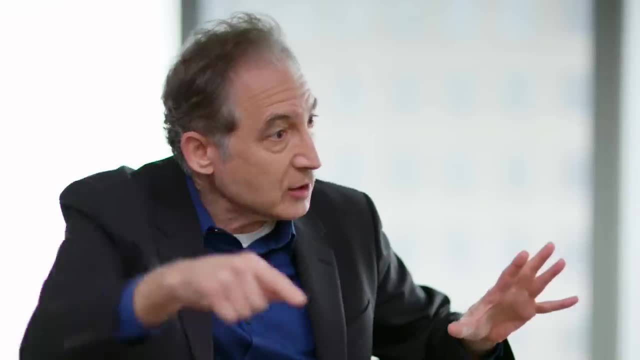 He showed us an approach to travel to the future. You want me to tell you how you do it. Okay, You build a spaceship, You go out into space really quickly, You turn around and you come back to planet Earth. And he showed us that when you're on that ship. 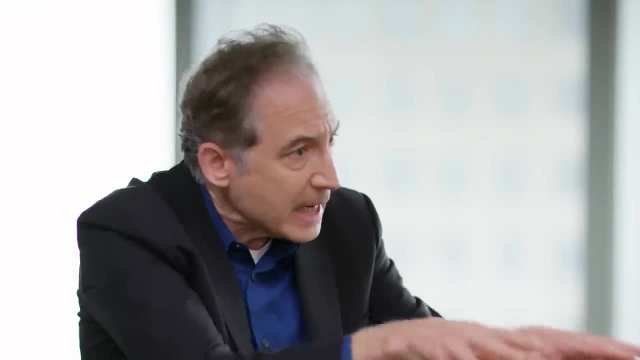 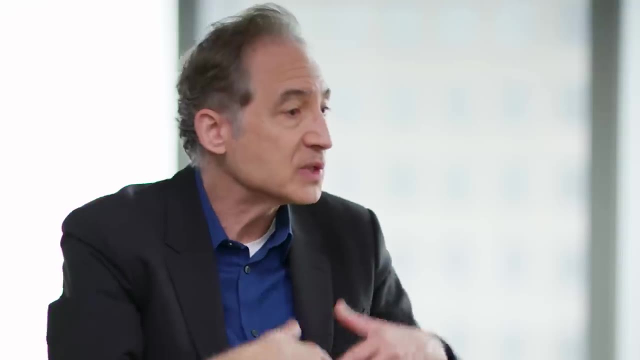 your clock will tick off time more slowly, You will age more slowly, So that journey may only take you, say, a year, six months out and six months back. But you know what, When you step out of the ship, it'll be a hundred years into the future. 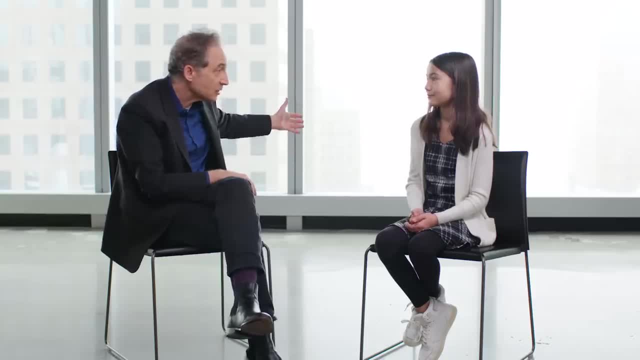 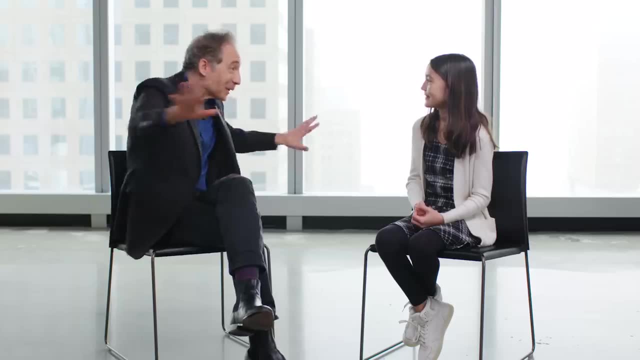 or a thousand years, a million years into the future. Would you do that? if you could, I would probably be dead by then. No, you'd be alive. That's the amazing thing. I'd be dead. Everybody else would be dead. 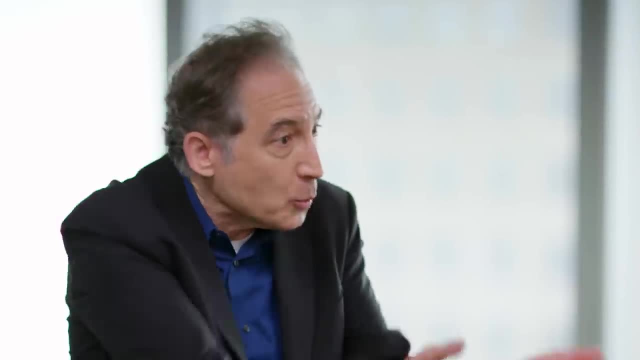 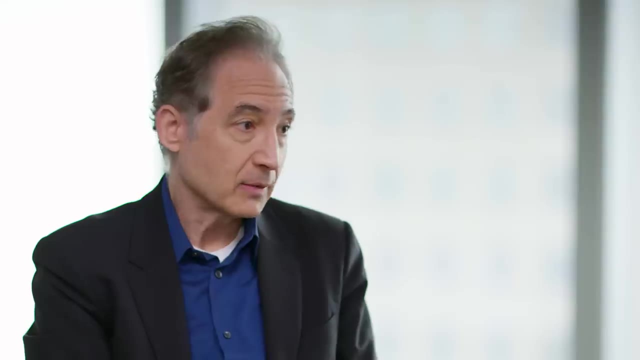 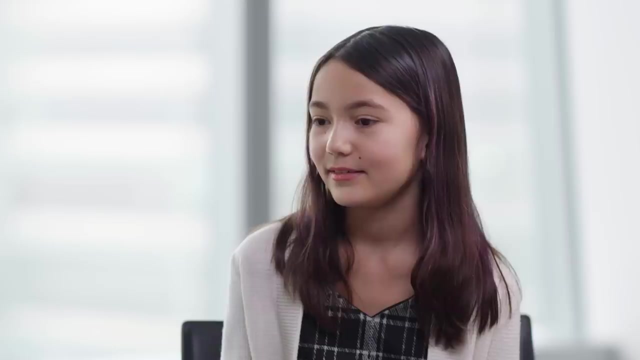 Who stayed on Earth, But your body would only age one year, and yet it would be a thousand years into the future. The question, though, is: could you get back? And I don't know the answer to that. Nobody does. We don't know if you can travel back, but we certainly know that you can travel forward. 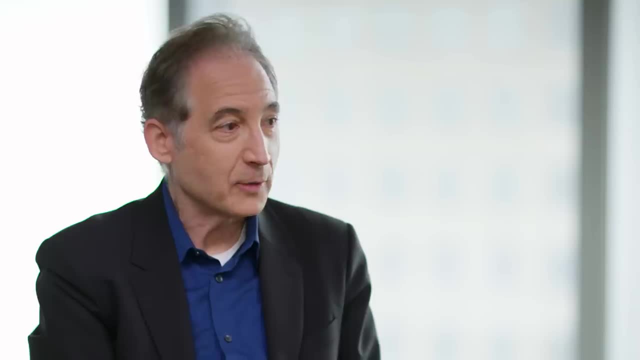 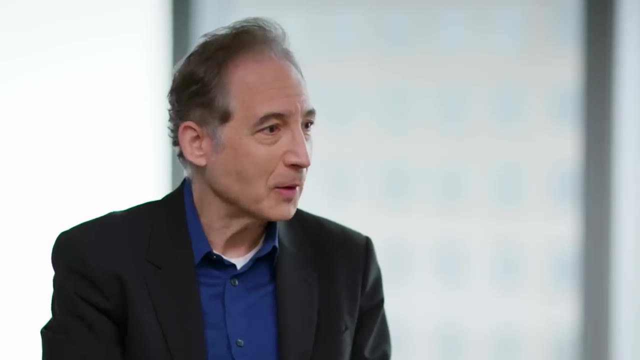 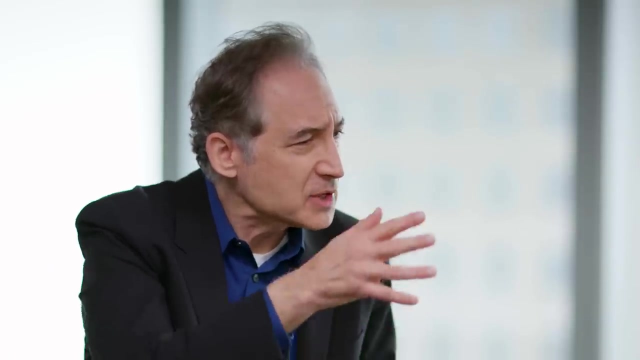 Has anyone ever tried to go forward and back? I don't think so. That same guy with the crazy hair, Albert Einstein, showed that there's actually a limit to how fast things can go. And you know what the limit is. The limit is the speed of light, Because light travels 671 million miles per hour. That is fast enough. 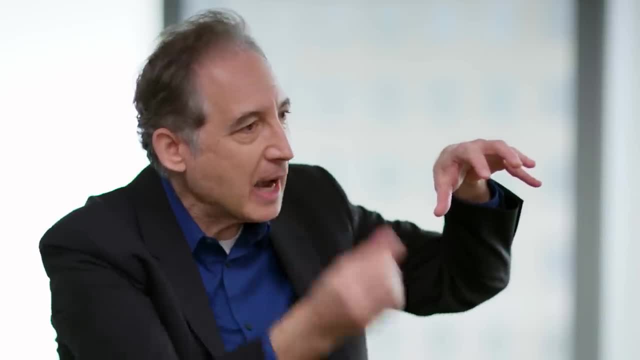 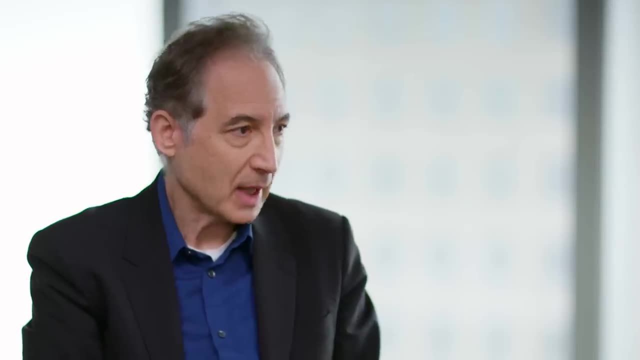 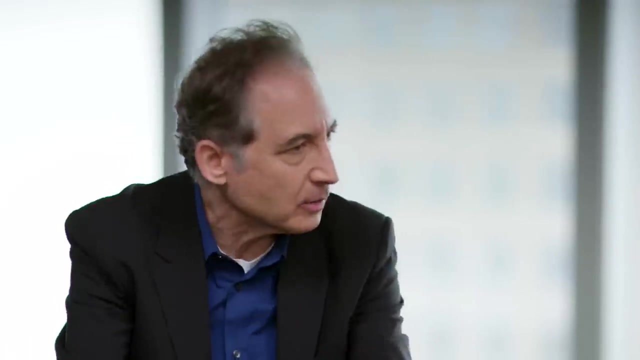 to go around the entire Earth seven times in one second. So if we could build a spaceship that would go as fast as light, we'd be able to do what Einstein noted. There's something else that's really curious about time. Things tend to go in one direction, and we call it the arrow of time. 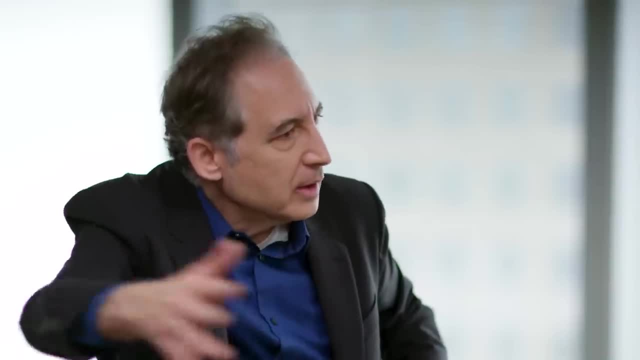 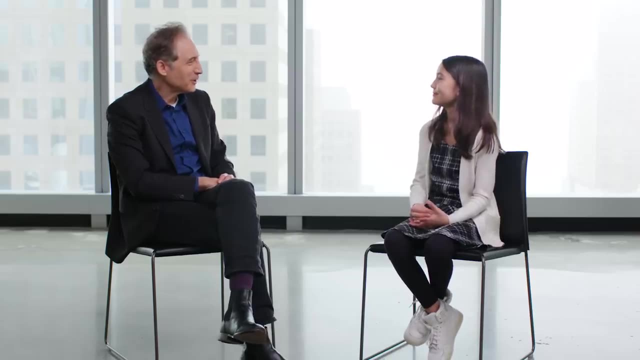 It sort of points from the past into what we call the future. If you were to ask me, why is there an arrow to time, Ask me, Why is there an arrow to time? I'm not really sure. I have some ideas, but I'd say we've still not completely nailed it down. 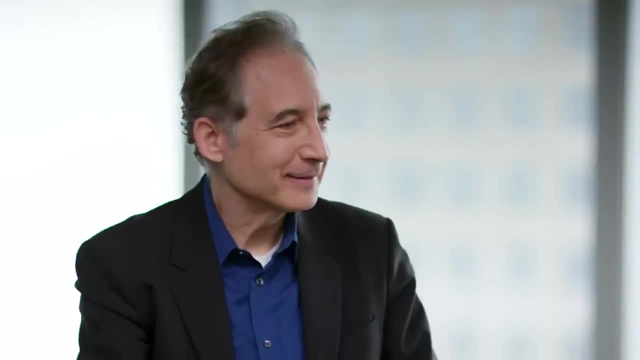 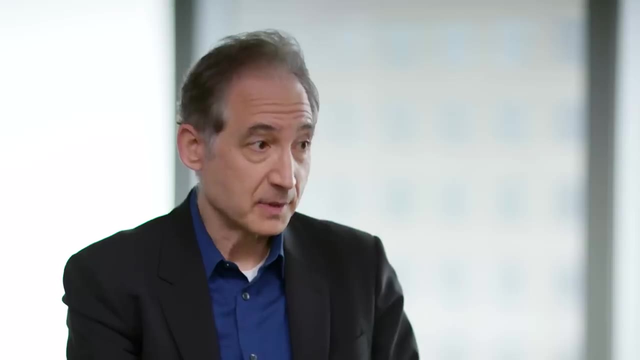 Kayla, what have you learned about time from talking about it here That you can't really travel back through time? And can you travel to the future? in principle, Maybe. Maybe That's absolutely right. I think it's unlikely. we'll learn how to travel to the past. 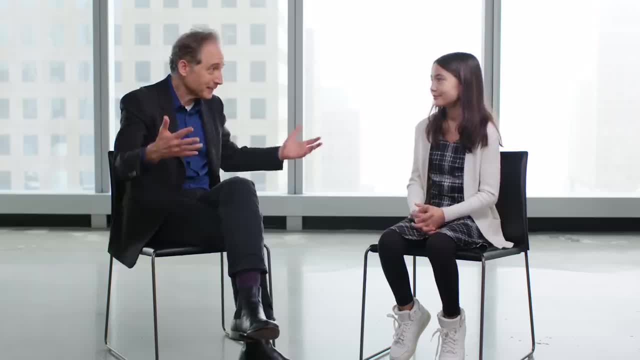 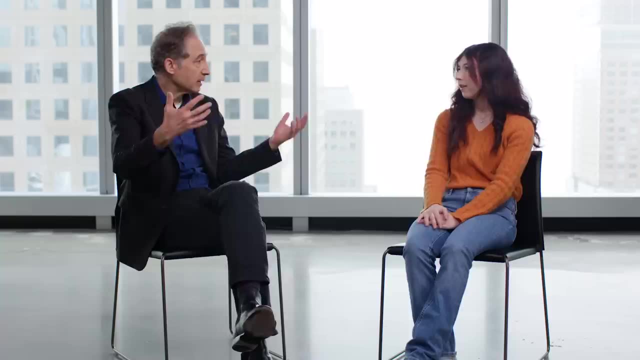 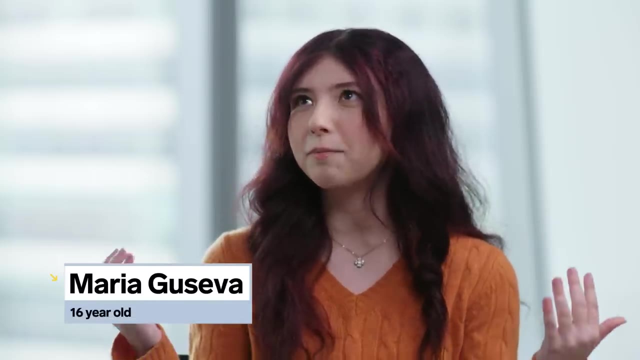 but it's not been ruled out. That's kind of exciting that it's still at least an open possibility. Yeah, What is time? If I was to ask you what is time, What would you say? Time is kind of strange because it's almost a man-made idea. There is the tangible of 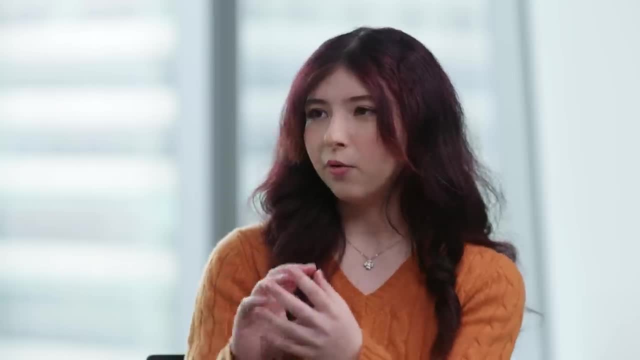 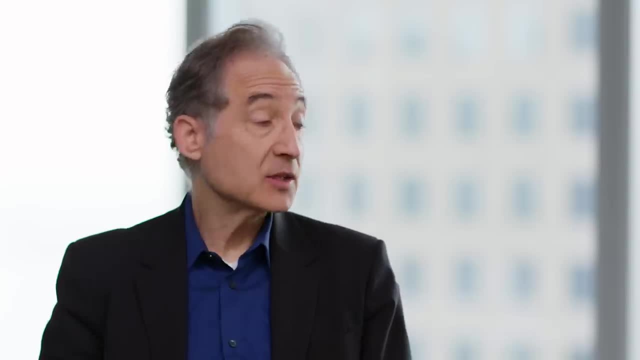 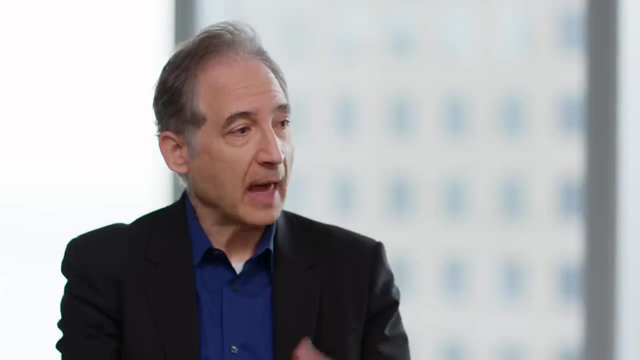 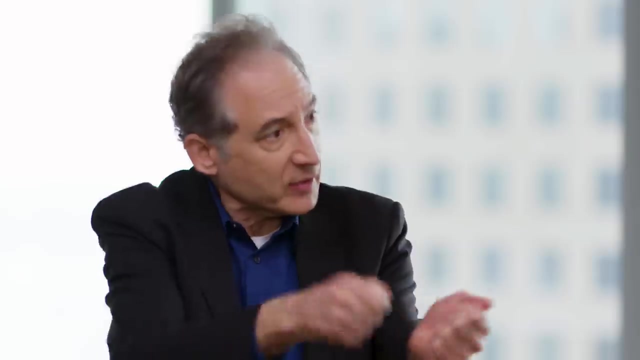 I think we all agree the universe existed. Did things change before there was life on Earth? Yes, And how would you talk about that change without invoking this concept of time? It's difficult to talk about something without adding time into it, Even if it is a human-made concept, that the universe evolved, developed, changed. 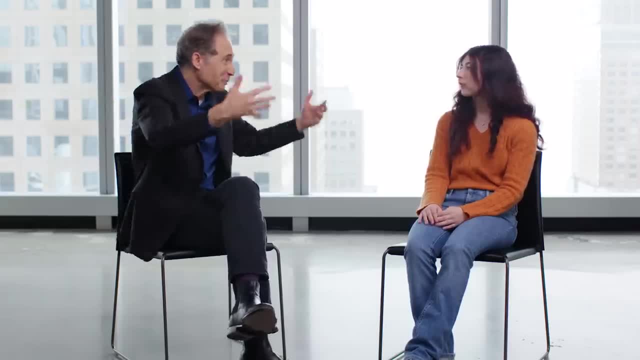 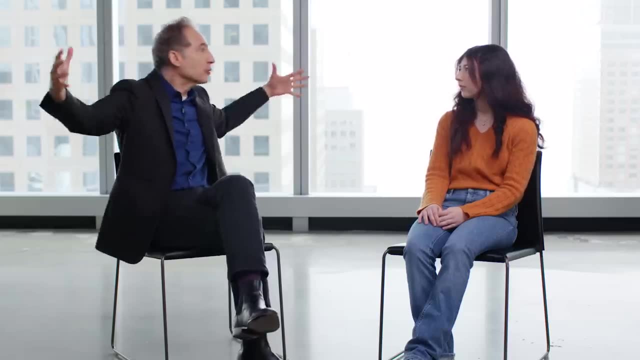 through time, ultimately giving rise to galaxy, stars, planets and, on this particular planet, planet, life. That conception of time gives a feel that it's like universal, that it's out there, It's the same for everybody, It's independent of our actions or activities. 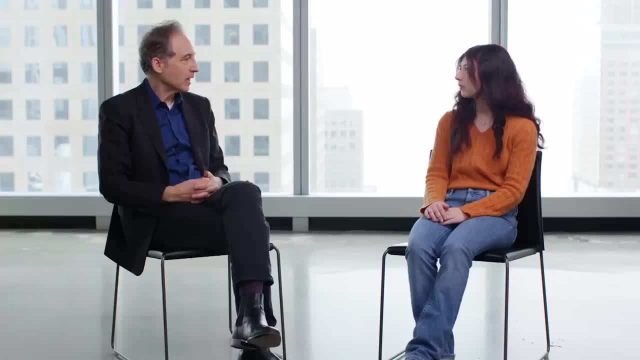 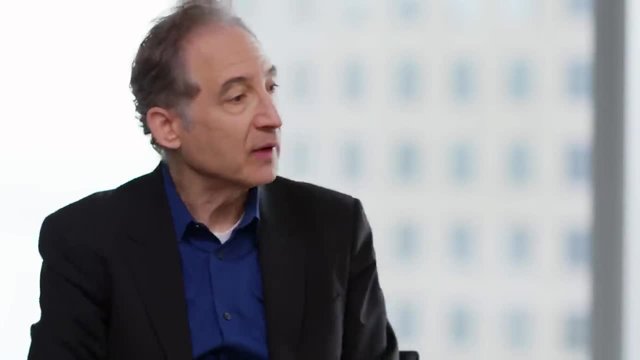 Do you know that Albert Einstein shattered that view of time? He found that if you and I say have identical wristwatches, I'm sitting still. I'm watching you move. I will find that your clock is ticking off time more slowly than my clock. 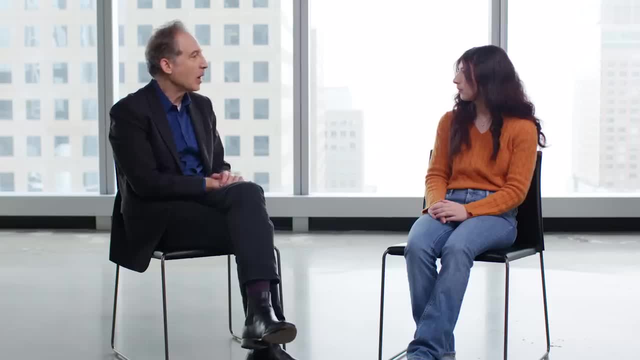 You know what's really remarkable. You can figure out This quality of time If you know one fact: that the speed of light is constant. Have you ever heard that phrase My freshman year of physics class? Yeah, If you're clever you can use that with high school algebra, maybe even a little high school. 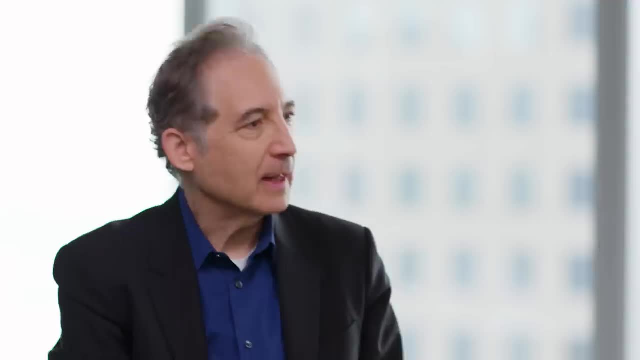 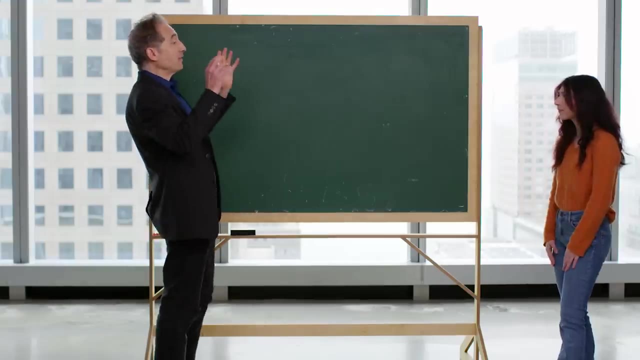 trigonometry to make it even easier to derive that clocks take off time at different rate. Do you want me to show you how that goes? Yes, please. All right, So to figure out the effect of motion on time, I'm going to use a really simple clock. 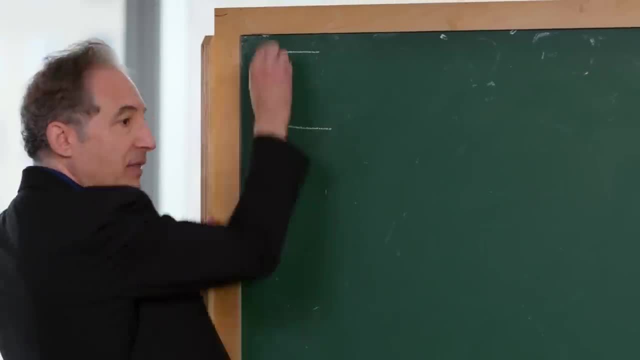 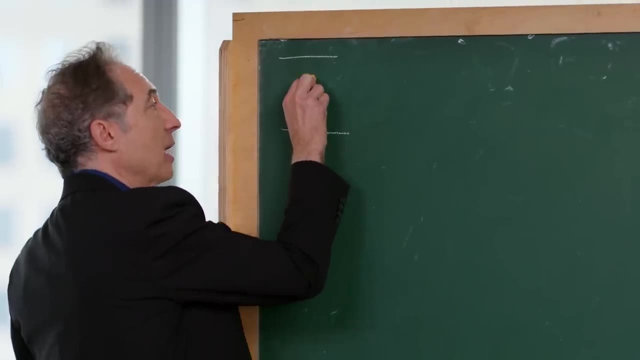 It's called a light clock. It's two mirrors that are facing each other And what we do is we have a little ball of light called a photon right That goes up, hits the top mirror, then comes back down and hits the bottom mirror. 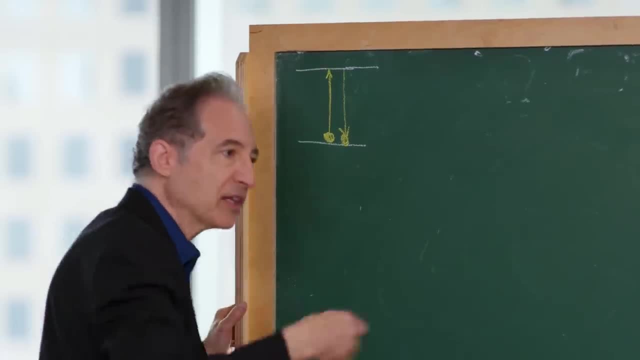 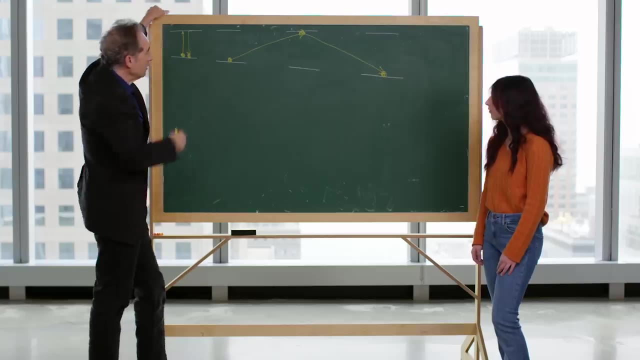 And every time it does that you go tick, tock. That's one unit of time. Imagine now we have another one of these light clocks, but I'm going to have it in motion Now. what do you notice about that path? 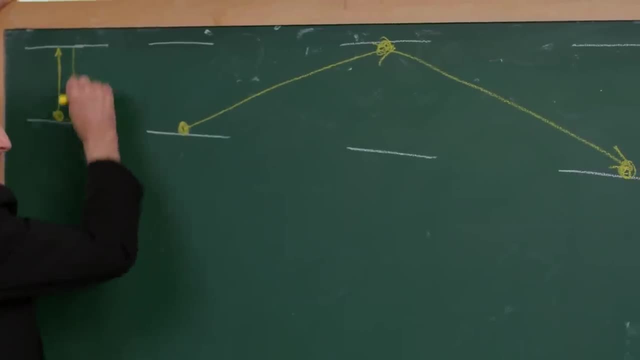 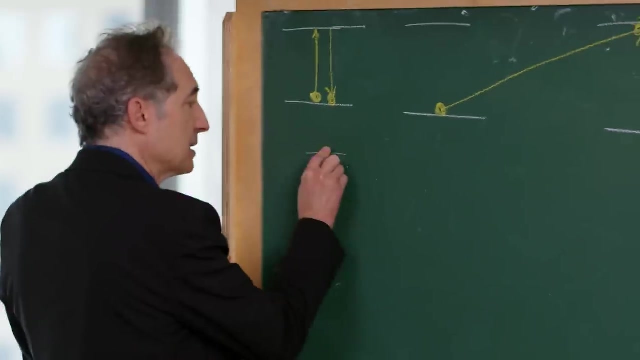 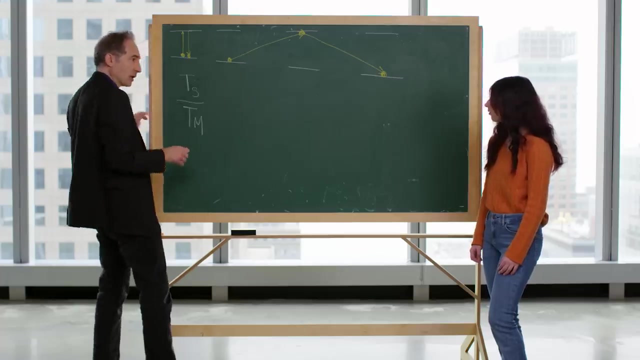 It's much longer. It's much longer, right, This one's going tick tock, tick tock. This is going to go tick tock. In fact, we can figure out the ratio. Let's consider time on the stationary clock compared to time on this moving clock. 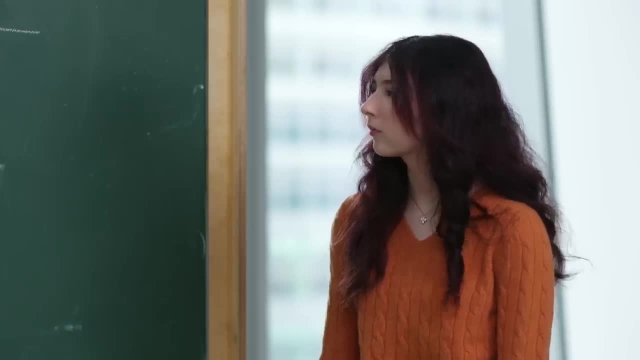 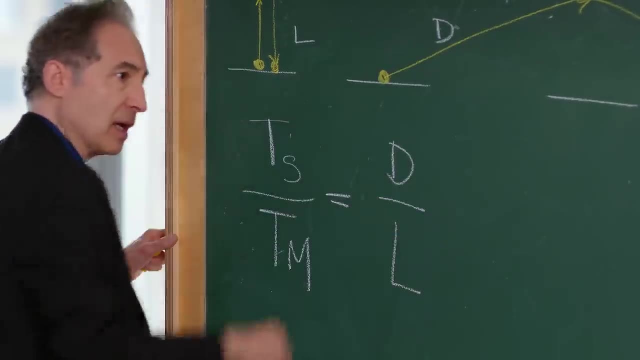 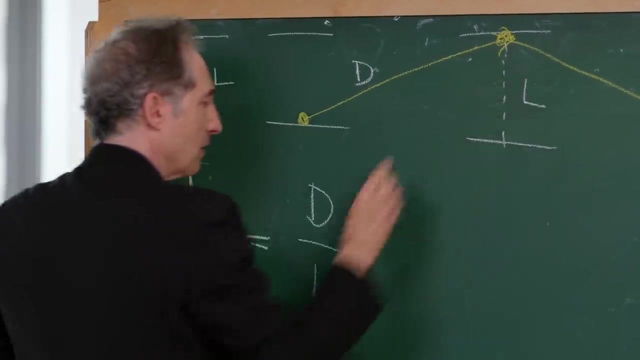 Well, that ratio is going to be the ratio of the lengths. Then this would be given by d over l- More time on the stationary because it's longer distance on the moving clock. Well, this length over here, that's the same as this l over here, right? 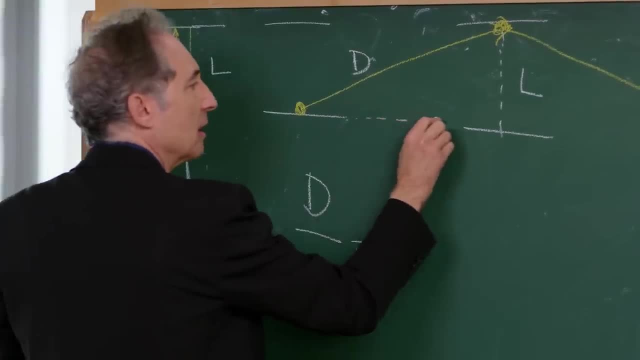 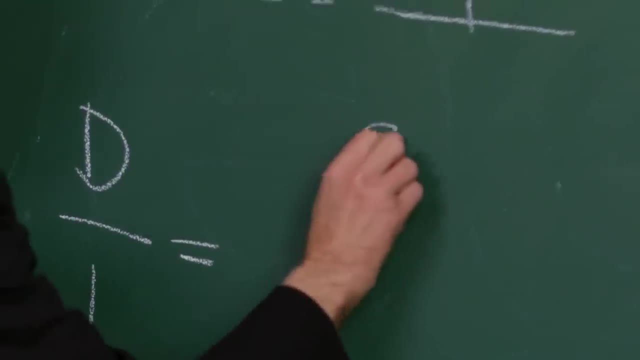 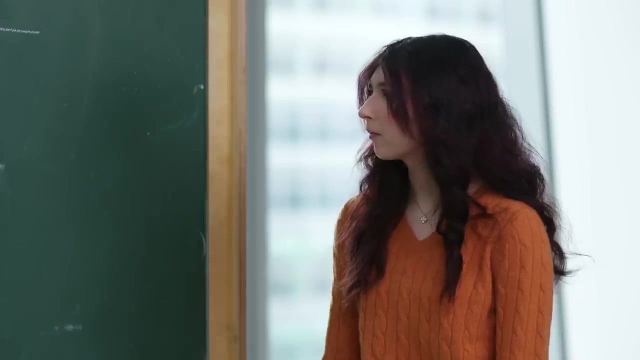 So we want d over l. Now you may recall that in trigonometry there's a name for l over d Sine of theta. opposite is l. Hypotenuse is d right, And so this ratio is just 1 over sine of theta. 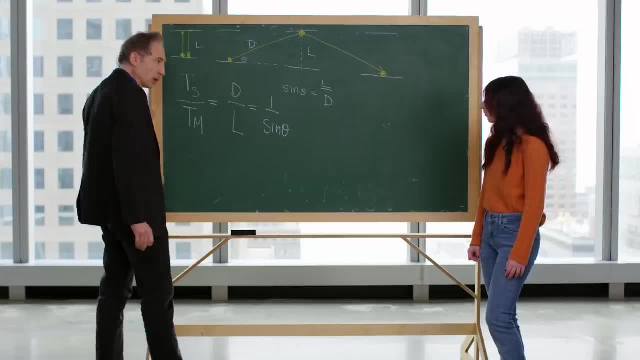 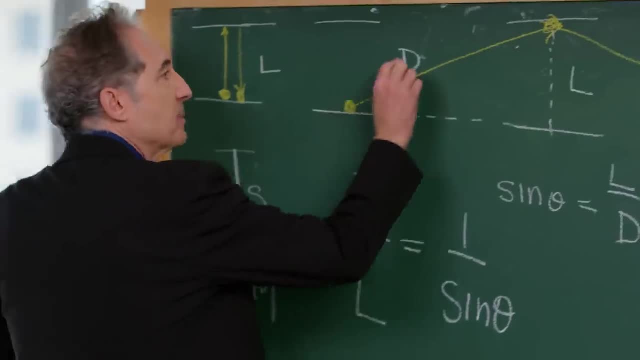 So if we can figure out 1 over sine theta, we'll have our beautiful formula for the ratio of time on the stationary clock to time on the moving clock. We just need one other fact: The speed of light along this diagonal is equal to what we call c. 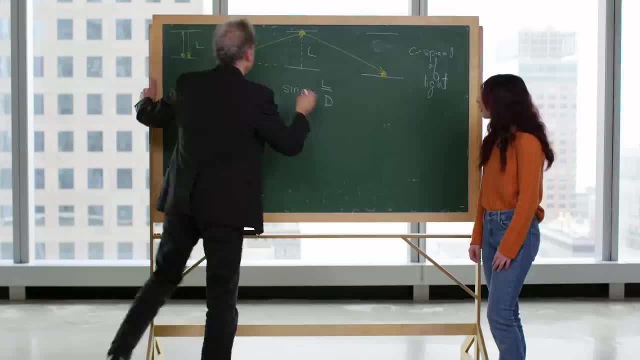 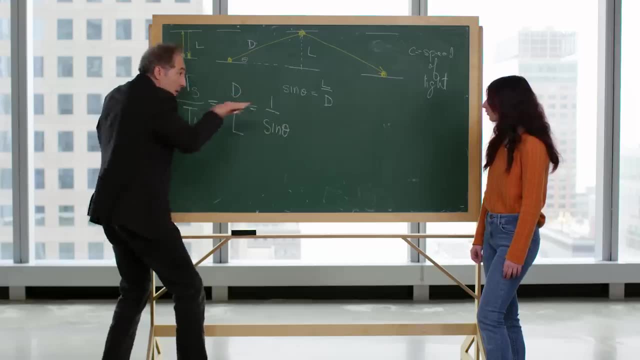 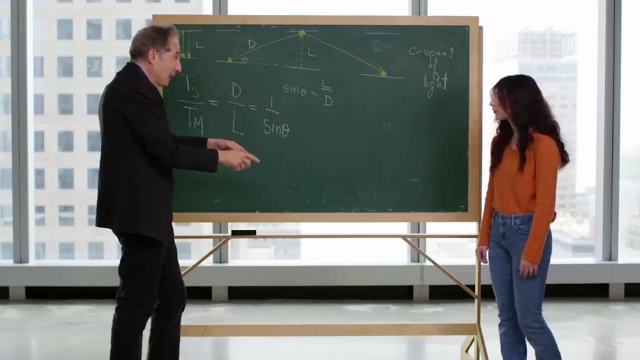 c equals speed of light. But in order for this ball of light to hit that point on the mirror, the component of the speed of light in the horizontal direction better be keeping perfect pace with the speed of the clock itself. So let's assume that this clock is moving in this direction with the speed equal to v. 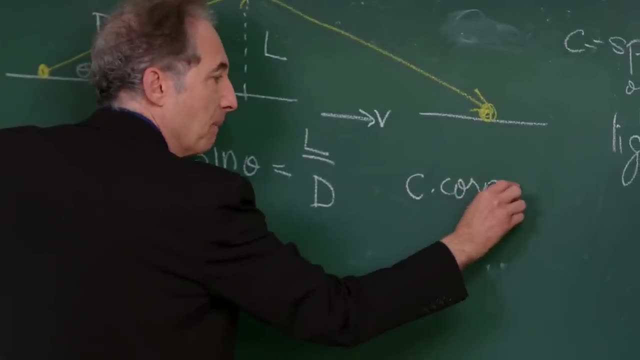 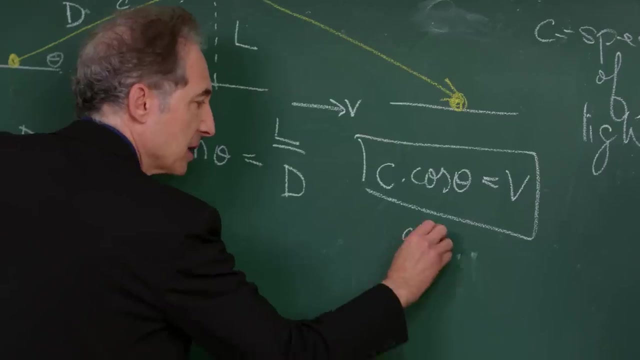 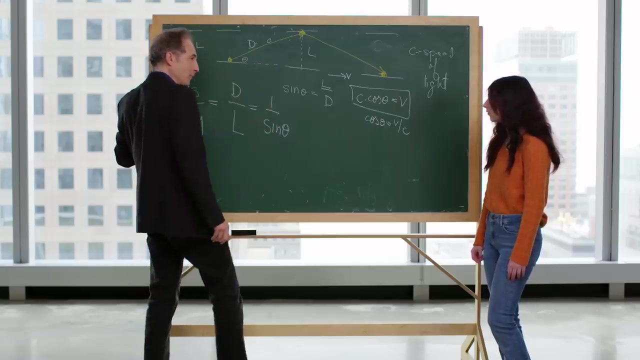 So c times cosine theta must be equal to the speed of the clock in motion, And from this we learn that cosine theta is equal to v over c. There's another beautiful identity you may recall from your study of trigonometry that you can use to calculate the speed of light on the moving clock. 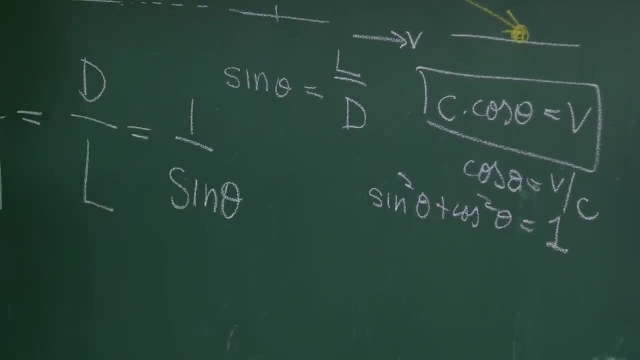 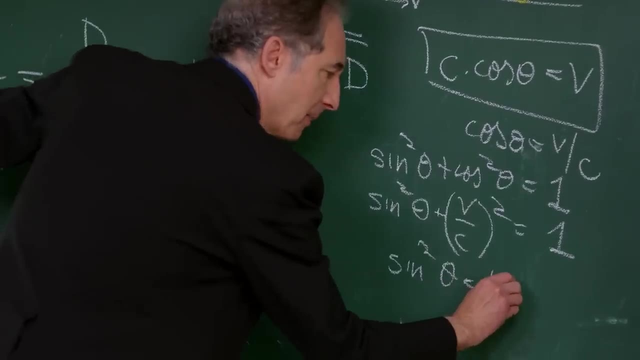 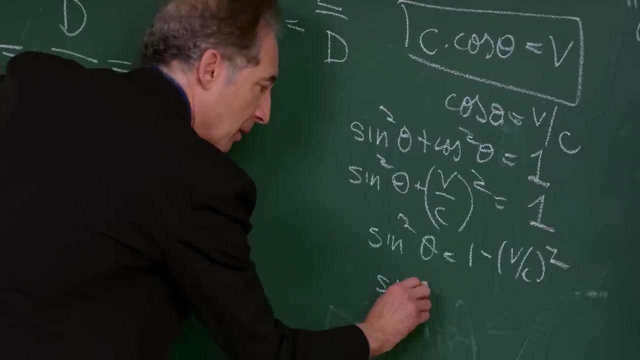 So if we take cosine squared theta plus cosine squared theta is equal to 1.. This is really just a Pythagorean theorem in disguise, And from that we can now solve: for sine squared, theta equals 1 minus v over c squared, And then for sine, theta is the square root of this. 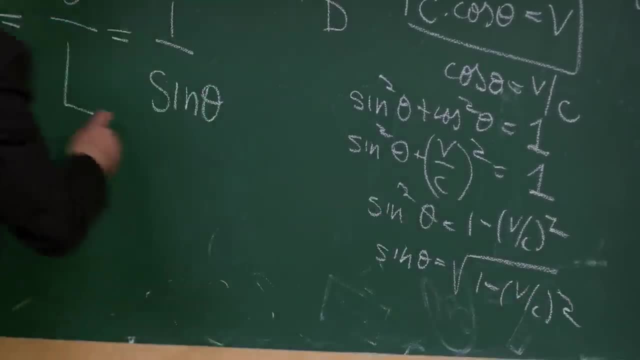 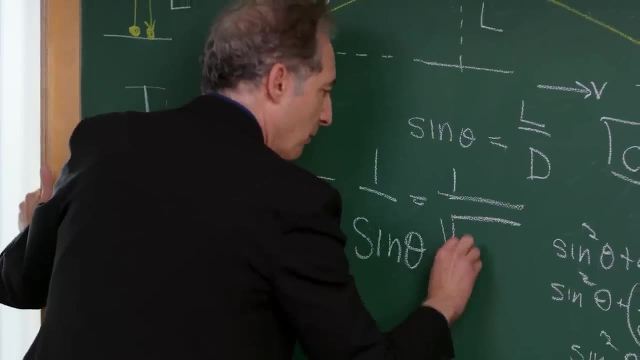 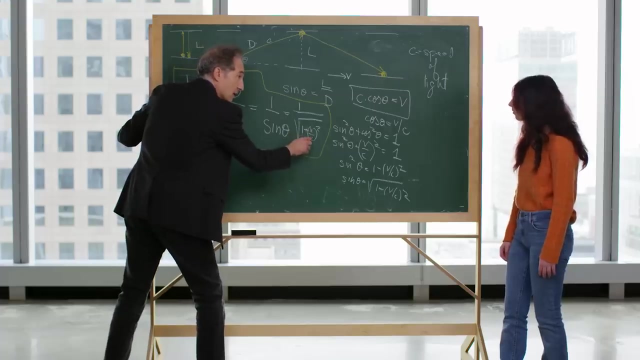 And now we're basically done, because we already had over here- that this ratio is 1 over sine theta, which is 1 over the square root of 1, minus v over c squared. So you see, as v gets very close to c, this gets very close to 1.. 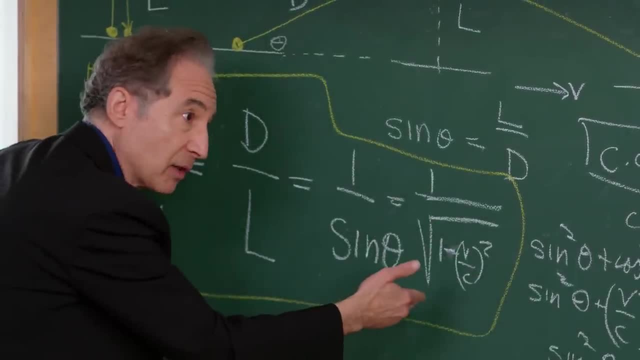 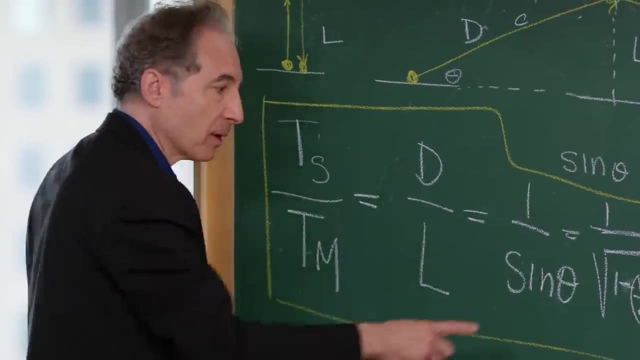 1 minus something very close to 1 is very close to 0.. 1 over something close to 0 is huge, which means the ratio of time in the stationary to time the moving. that can be a huge number as the speed of the moving clock approaches the speed of light. 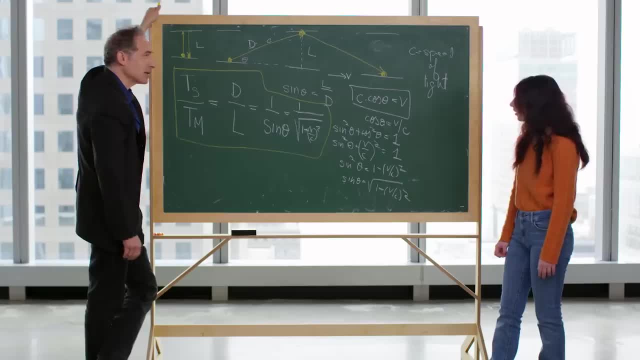 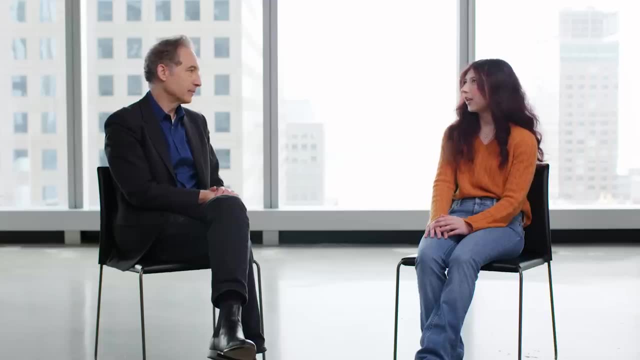 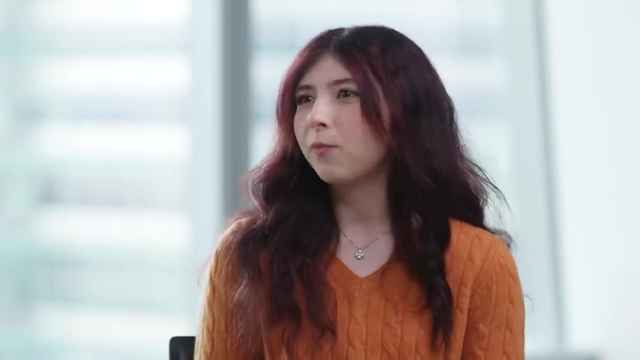 a light clock, but it's true for any clock, and this is what Einstein discovered in 1905 with his special theory of relativity. Do you think that in the near or foreseeable future of humans as we know ourselves now will there be a time where we are using these formulas and these concepts in our daily lives? 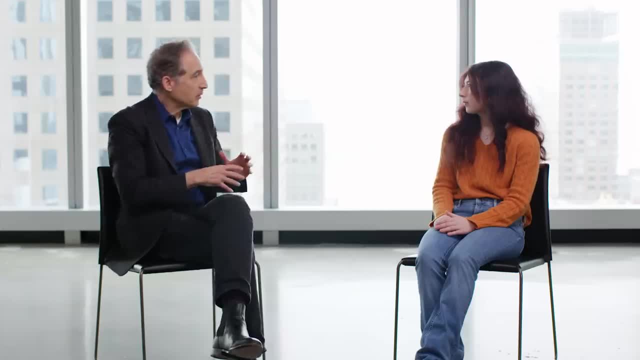 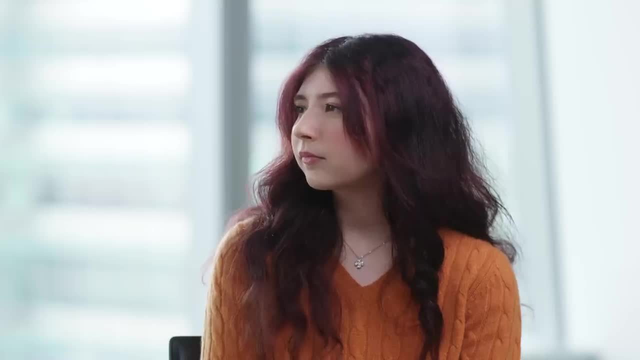 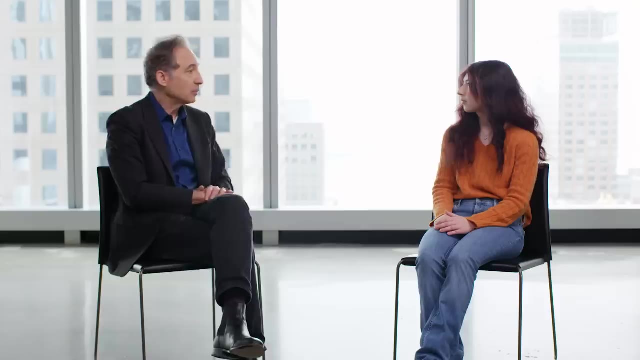 As technology progresses, the barrier between the limitations of experience and the truth of how the world behaves in extreme environments will be moved. In the very same way that you know we can toss a pack of gum and we know where to put our other hand to catch it, will we have that kind of intuition about these ideas? 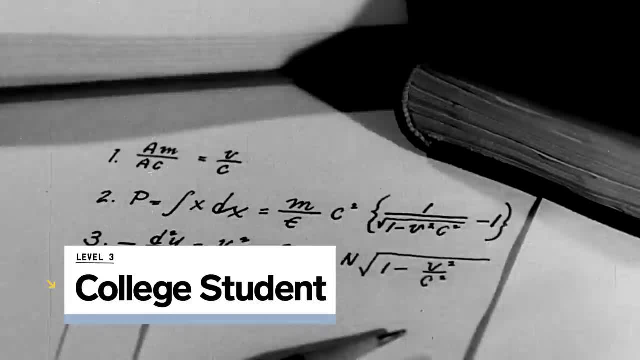 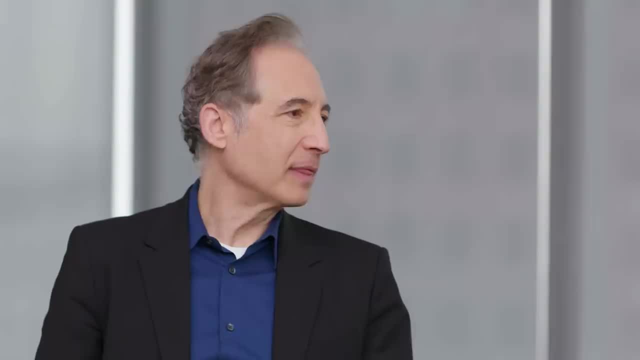 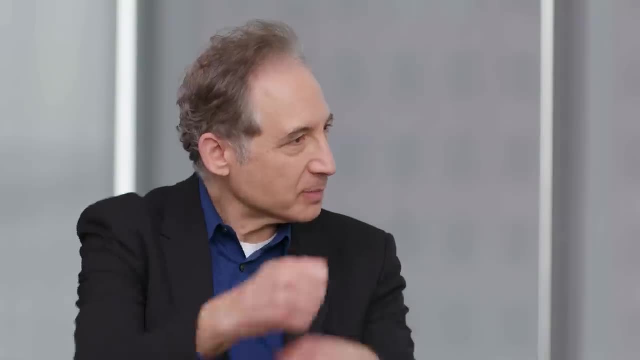 I think it's quite possible. What are you studying right now? I'm doing physics and computer science. So have you spent any time thinking about this weird quality of the laws of physics: that there's no mathematical distinction in the laws Between forward in time and backward in time? 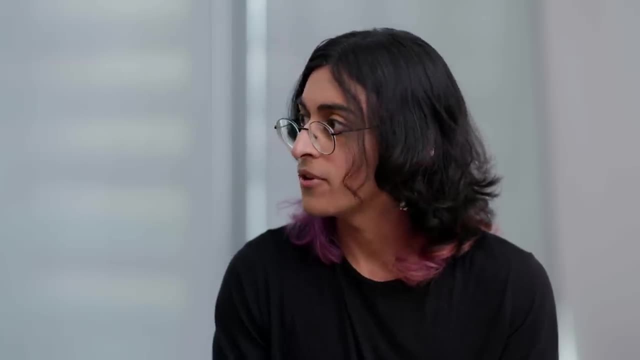 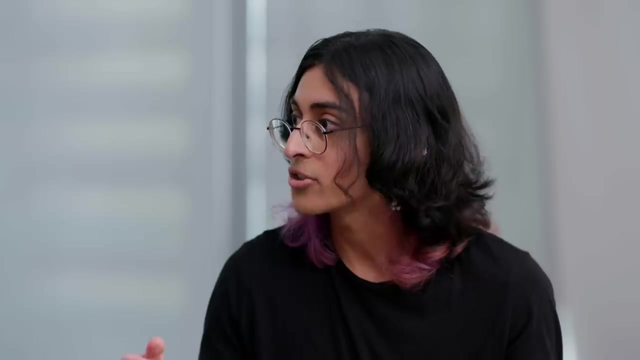 Is that something you're familiar with? Yeah, and the one thing that really confuses me- there I'm thinking about one of the most basic things we learn, I guess, from interstellar- is that the universe is expanding or space is expanding. 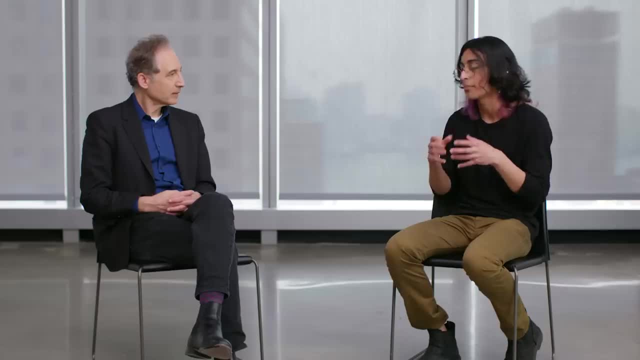 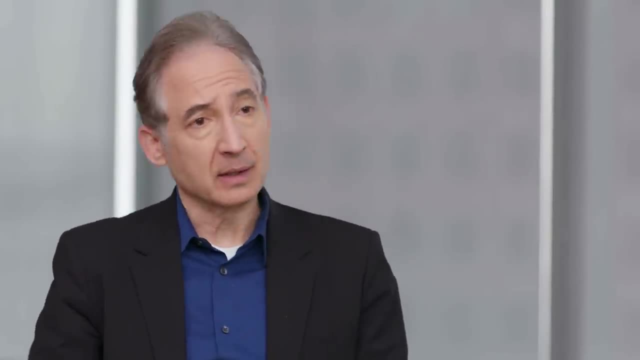 And so I'm thinking: how does that square with gravity and electromagnetism, which is like kind of predicated on the density of charges or masses? The fact that space expands is perfectly compatible with our understanding of all the forces of nature, Because all of them continue to operate. 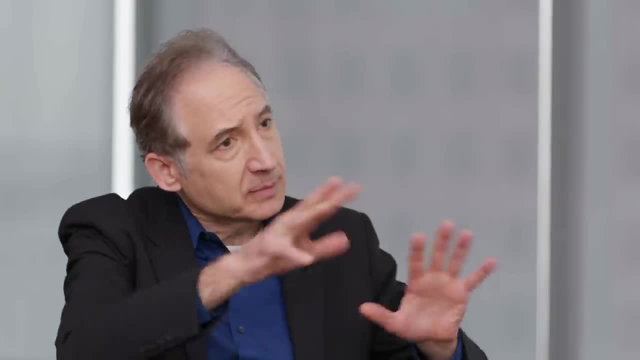 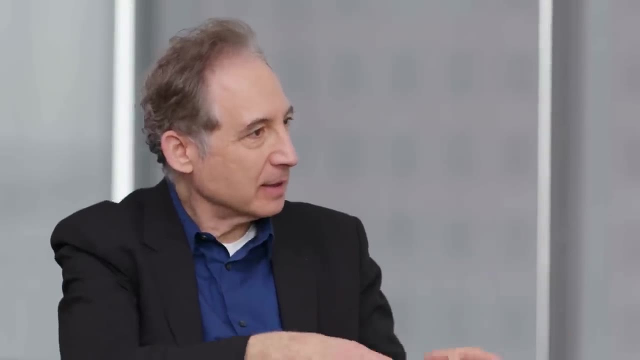 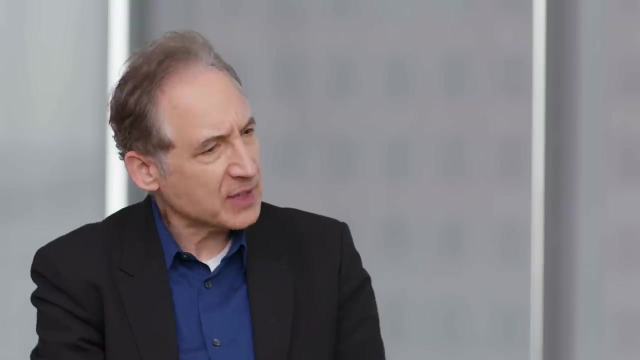 In a somewhat more subtle way, but we have a beautiful prescription for taking any law that we understand in the simpler context- a flat spacetime- and juicing it up so that it works in a curved spacetime. The more philosophical question is: in any of those formulations, if you replace t by 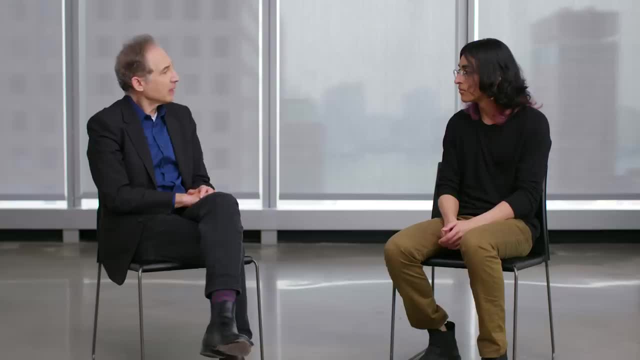 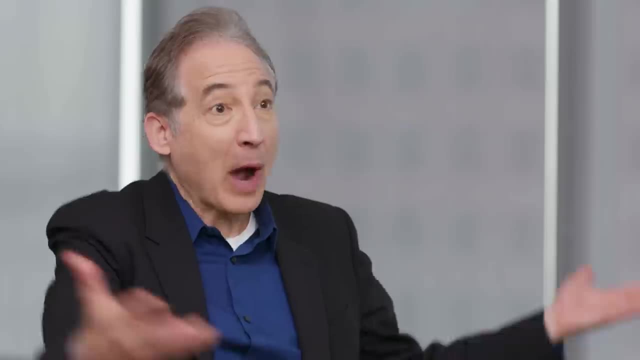 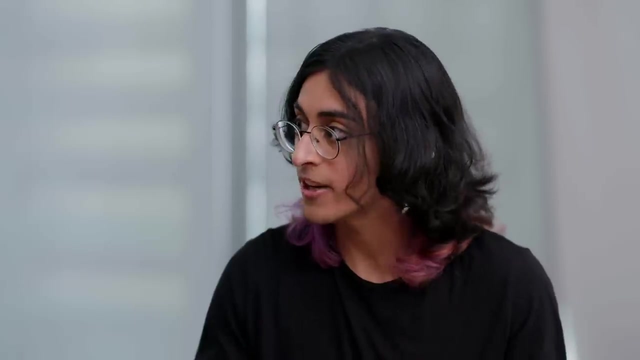 minus t and you do it properly in the equations. the equations still work. But if past and future are kind of treated on equal footing In the fundamental equations, why are they so different from the perspective of experience? When you're talking about the perspective experience, is that just human subjective? 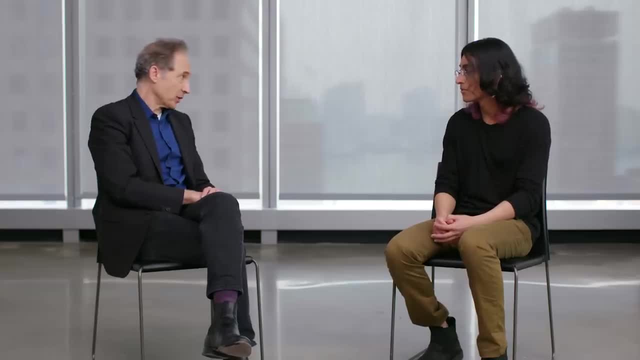 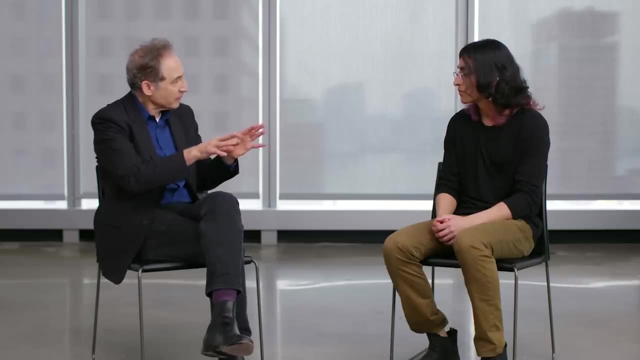 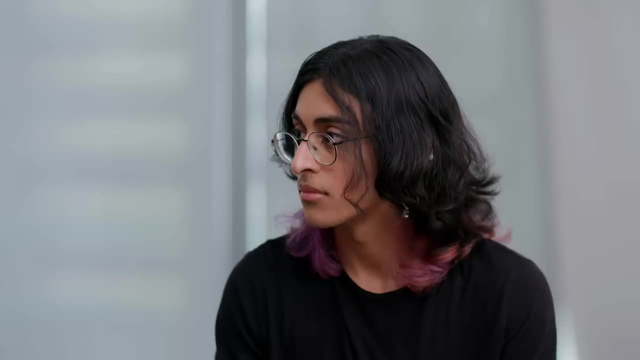 experience or actual observation for physics? Well, certainly it starts with human subjective experience, but then we are able to elevate it to a more objective description, For instance when we introduce words like disorder and order and entropy and the second law of thermodynamics. 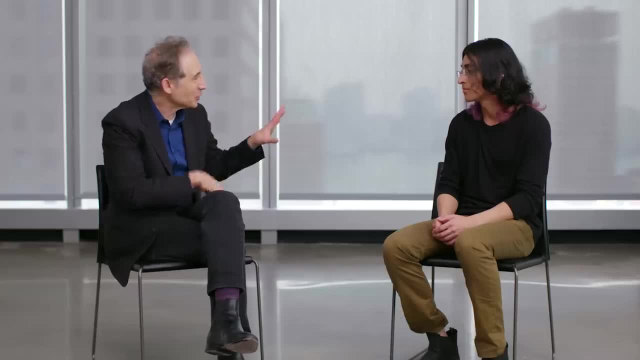 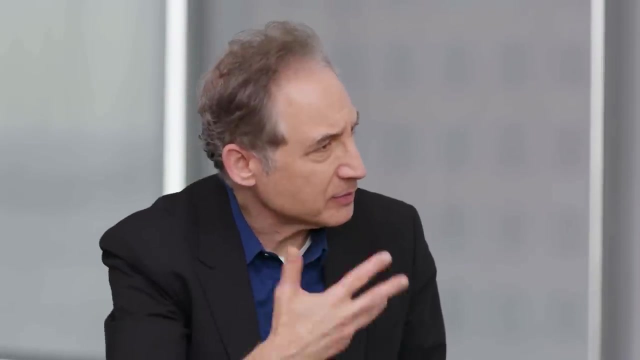 Usually the way we say it is: s equals k log w. Entropy equals Boltzmann constant times log of a particular quantity, which is ultimately counting the number of distinct configurations that a system can be in. What Boltzmann and others showed is that entropy tends to increase toward the future. 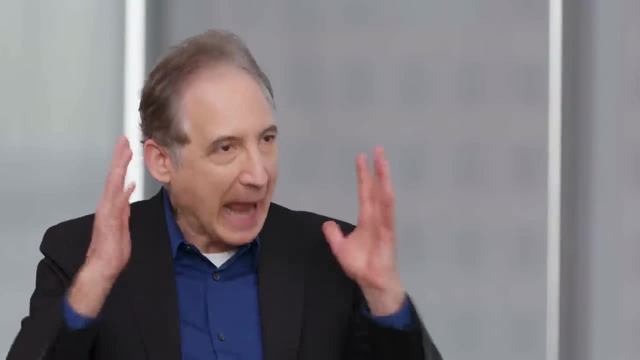 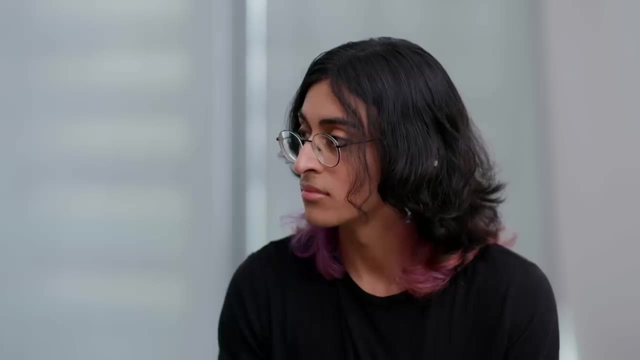 But the key word there is tends to increase. So this arrow of time Going from the past to the future rests on a curious foundation. It's a statistical foundation which says that it's more likely for eggs to splatter than unsplatter. 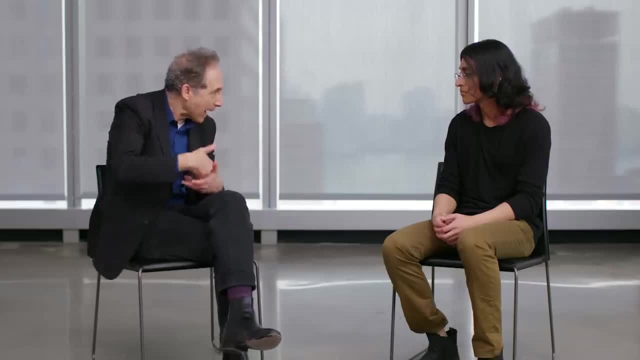 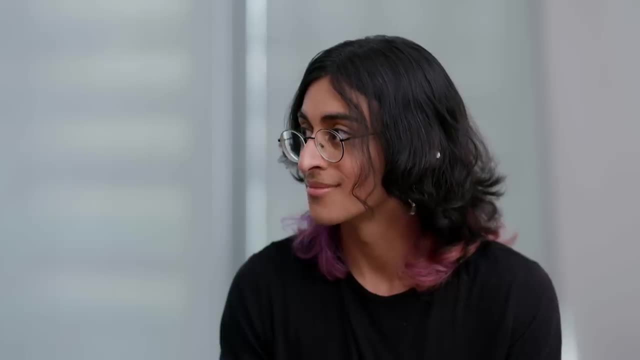 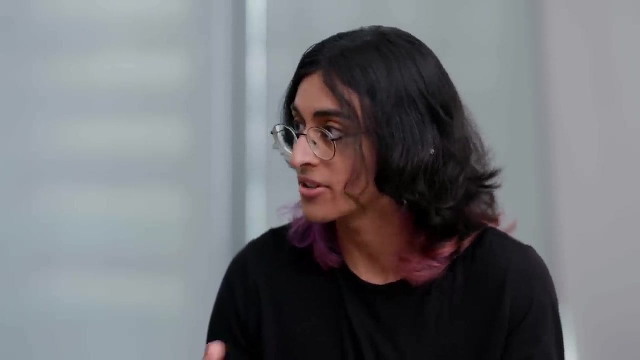 It's more likely for glasses to smash than unsmash, But not that it's impossible for these things to happen. You just have to wait a really long time for there to be a reasonable chance of it ever taking place. When you said that you know it's more likely for an egg to smash or for glass to smash, 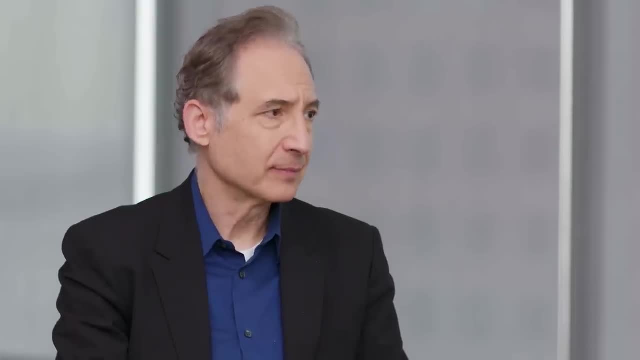 Probably because there's so many atoms, so much stuff going on. Yes, But I'm thinking, if we zoom in on like a single thing, I guess do we have variations that are extremely unintuitive, because you know things can happen in a way that isn't. 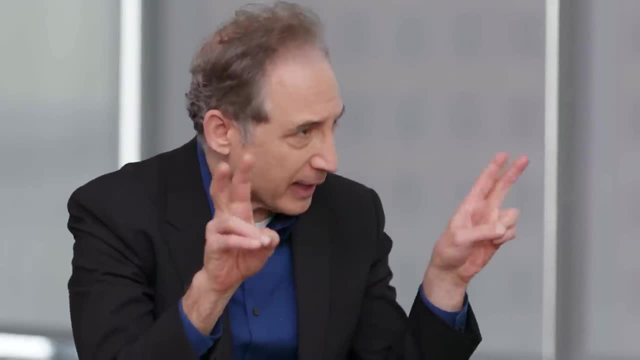 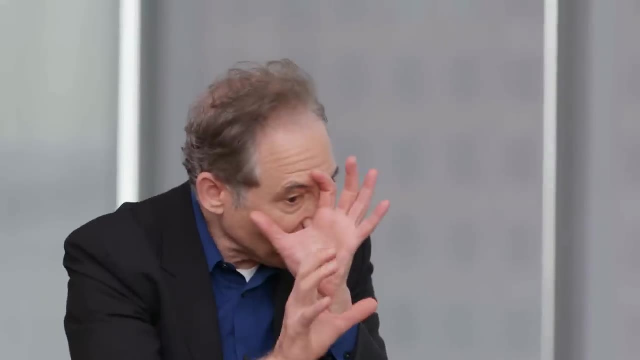 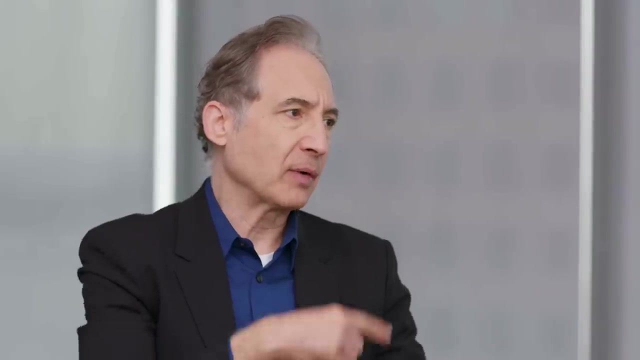 a statistical average. If I take a film of that electron- and it's a little fanciful to describe it that language because you know about quantum mechanics and so forth- but I take a film of a little particle moving around and I show you that film, you'll be really hard pressed to determine whether 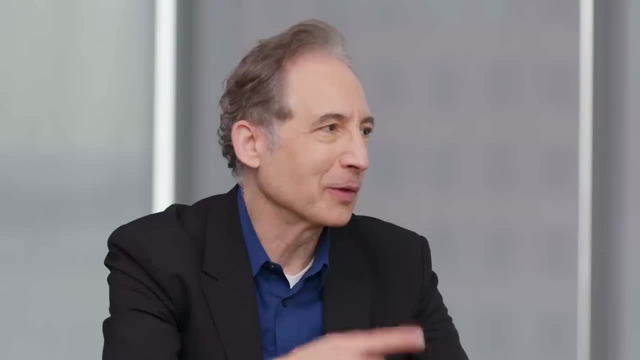 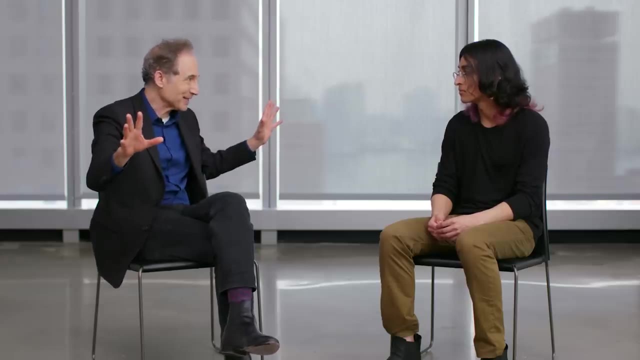 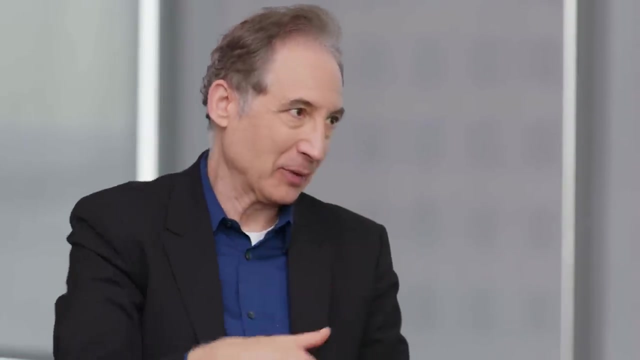 I've shown you the film running forward in time, Mm, Or whether I've shown you the film going in reverse time. If I had two or three or four or a gazillion particles into the mix, then it will be much easier for you to determine whether the film is going forward in time or backward in time. 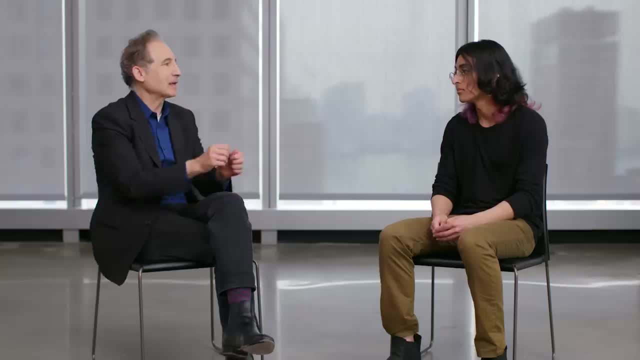 But order and disorder don't have much meaning if there's only one particle, And that's why the fundamental laws don't draw a distinction, but the macroscopic experience does. But it raises a key question: Where'd the order of the egg come from? 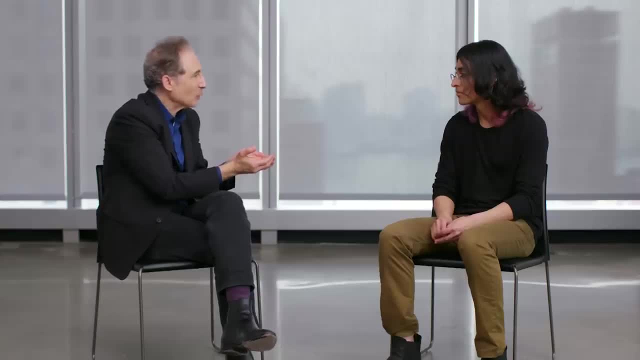 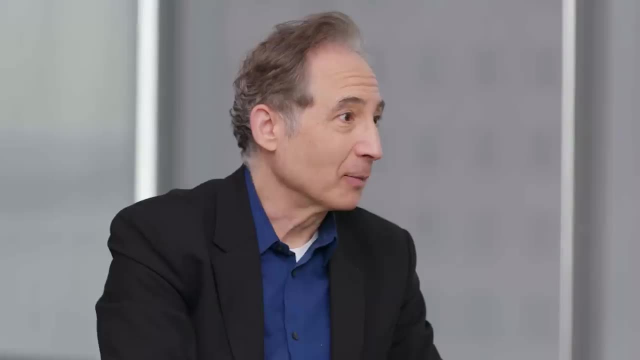 If everything's going in reverse time? what's the order of the egg If everything goes toward disorder? how did I get this orderly collection of atoms called an egg? Well, you probably would say from… Chicken, A chicken. But then I say to you: where'd the chicken come from? 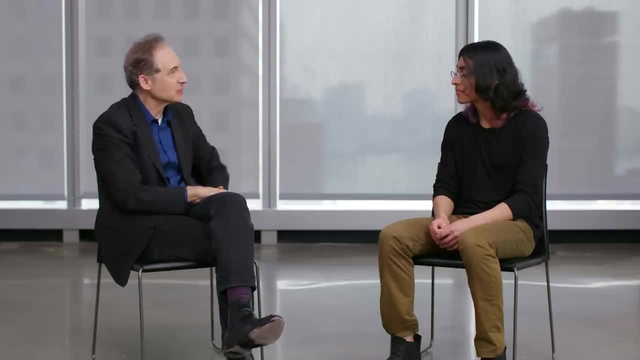 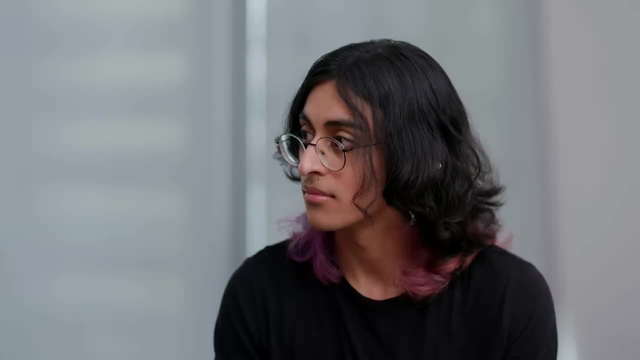 And you say from an egg. But there's actually some real insight we can draw from this because if we keep going back with the chicken and egg story, we'll go back through the evolutionary lineage of life, We'll go back to early moments of the sun and the galaxy and, ultimately, the universe. 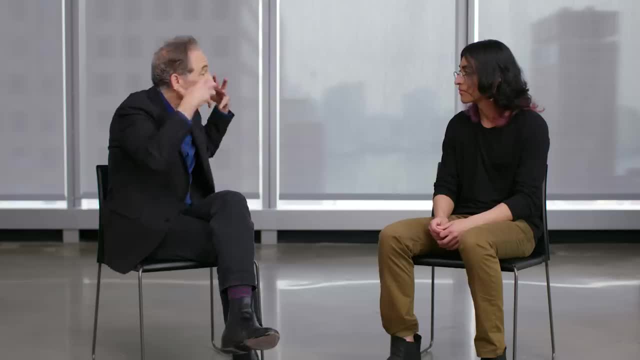 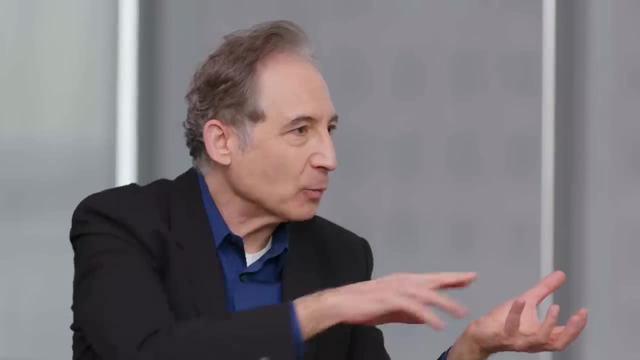 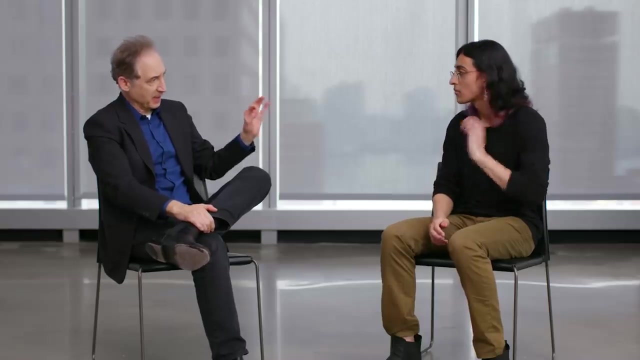 each step taking us to greater…, Yeah, …and greater order. So we believe that the ultimate source of order is the Big Bang, itself Highly ordered beginning, called the bang, And we have been living through the degradation of that order ever since. We still don't really have a solid explanation for why the Big Bang had to be or was highly. 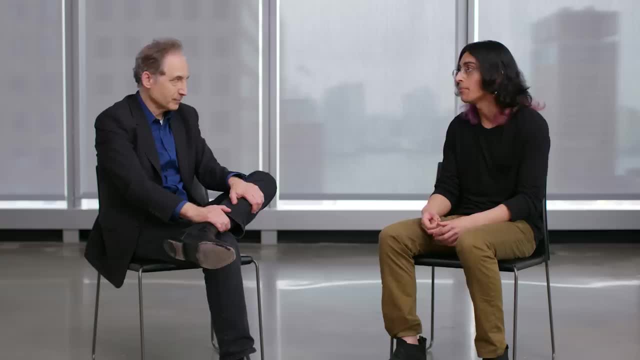 ordered. At the moment it's really a deep assumption. Back with Einstein we wondered: does time change with speed? And that's another change with that. Before we didn't think possible. but I guess we found out eventually Some of the fanciful ideas. 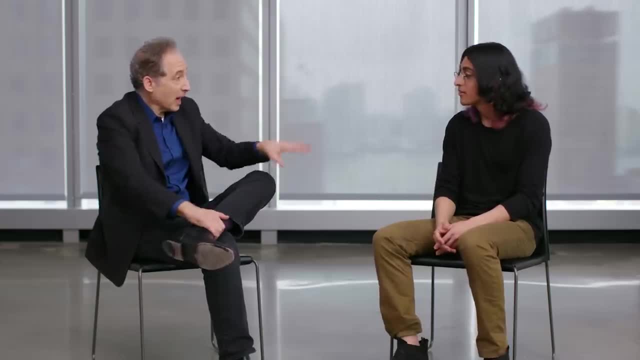 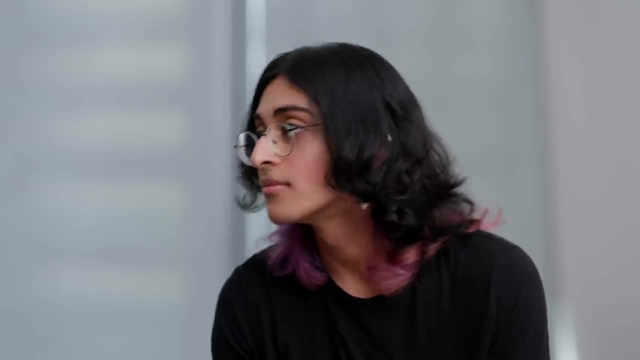 I guess it was a tiny sliver of hope there. Yeah, Not only did we find that time changes with speed in special relativity, but we also found that time changes with gravity. Einstein showed that the rate at which a clock ticks slows down based upon the stronger gravitational. 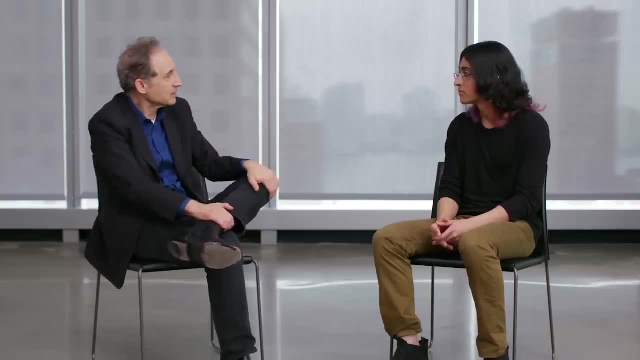 field or gravitational potential actually, that it is experiencing. I think you mentioned interstellar before. Do you remember the scene in Interstellar? Yeah, They go down to a planet that's near a black hole. They go down to the planet and they spend just a couple hours there. but when they go, 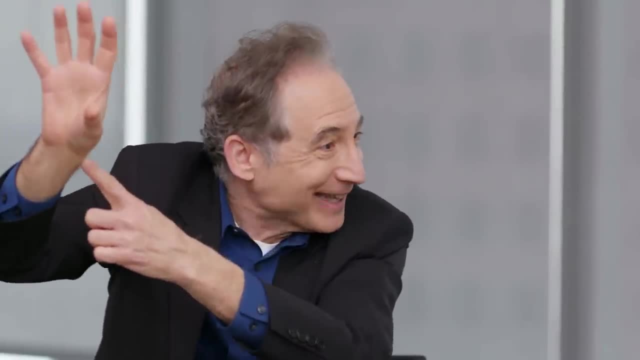 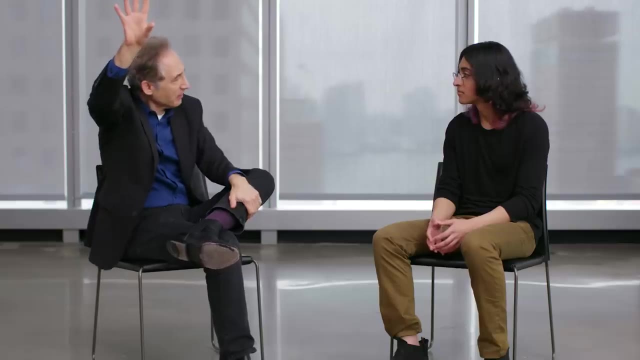 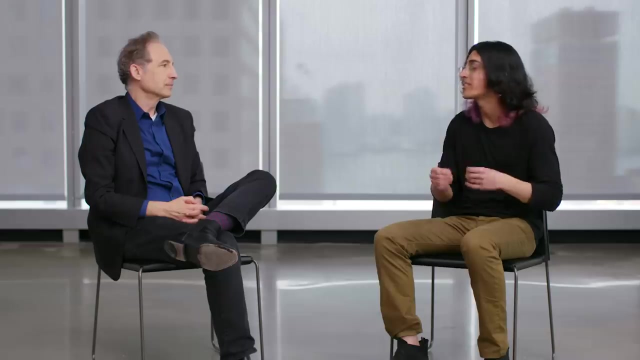 back to the ship. it's 23 years later on the ship because time is elapsing slowly near the strong gravitational field, comparatively quickly far away, And that's not science fiction, That's actually how time behaves. I've always heard people say: oh, general relativity, it might not seem applicable. 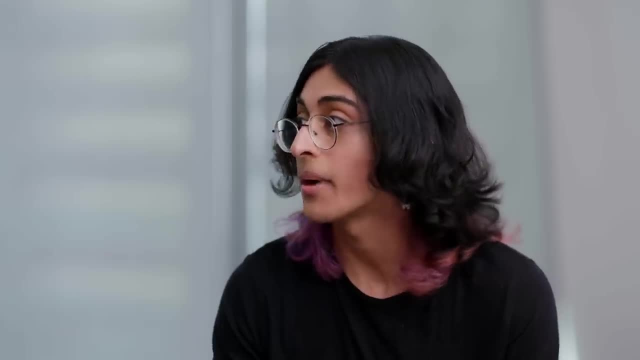 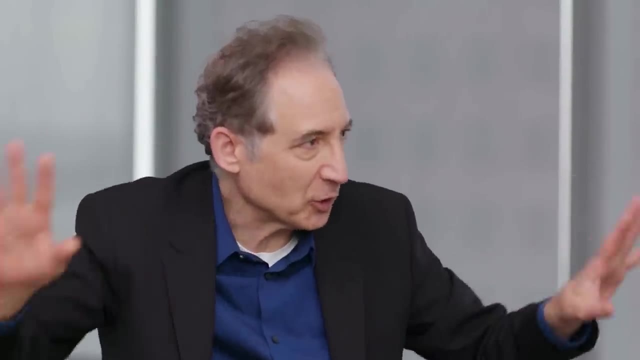 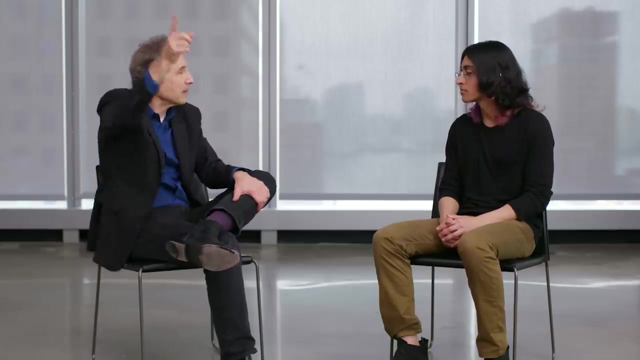 but GPS due to satellites. Yeah, You can't measure clocks by accounting for relativity, Well, but that's even a really, really good point. The GPS would become completely inaccurate in a very short period of time if the satellites weren't taken account of or the software wasn't taking account of the fact that time 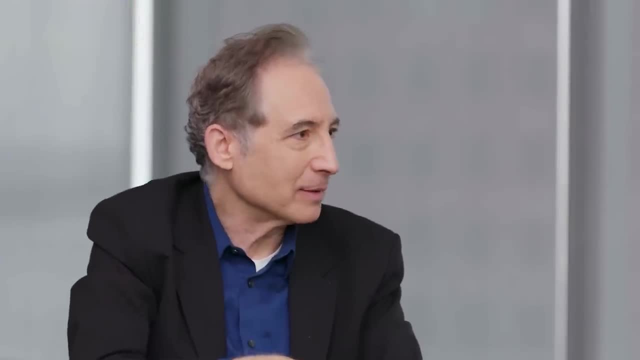 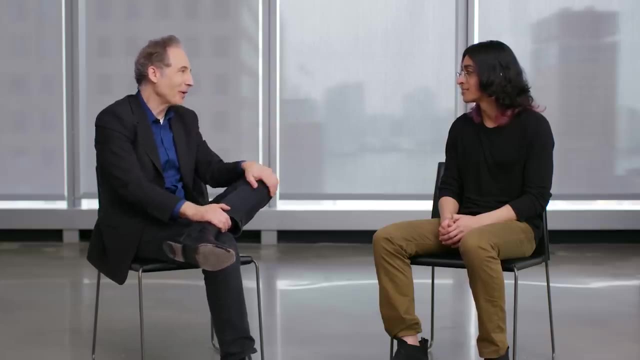 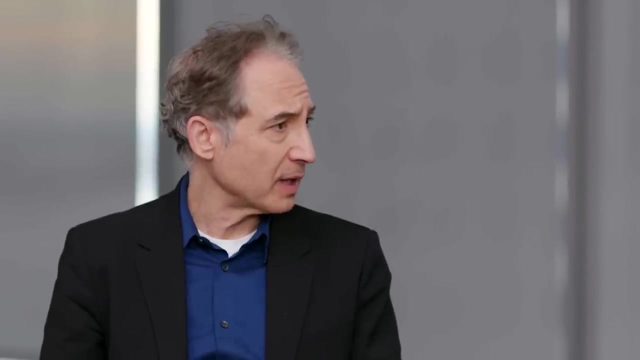 elapses differently for the clocks on the satellite compared to the clocks down here on Earth. So we walk around with general relativity in our pockets, even though most of us perhaps don't really know that. Have you started any projects yet, Or that's? 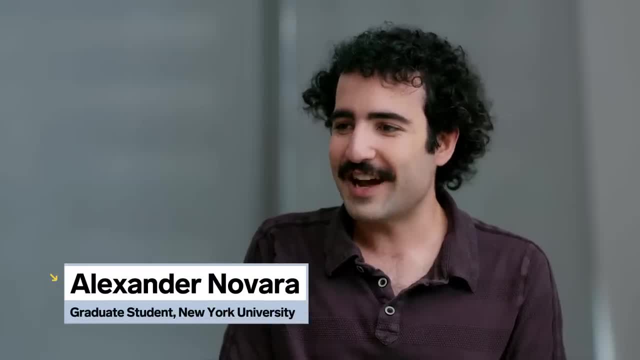 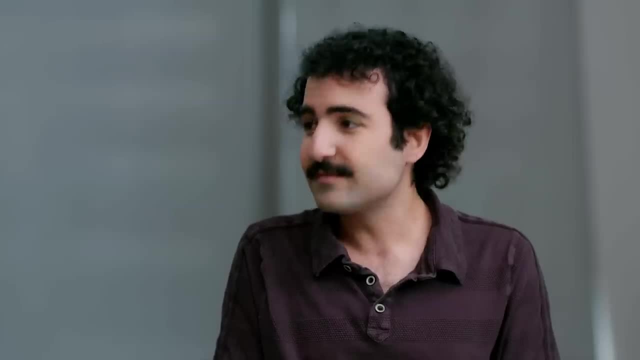 I'm just starting one right now. What's it on? I'm trying to figure out how stars in the galaxy are moving, based on what they're made of, which is interesting. Oh, Clearly, time comes in to what you're doing. 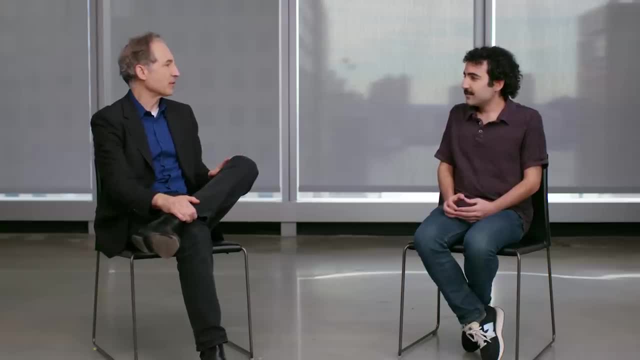 To what extent do you have to grapple with some of the subtle features of time? Yeah, with my research in particular, I really want to know what happened in the past and what happened in the future, but you only get a single snapshot when you look up at 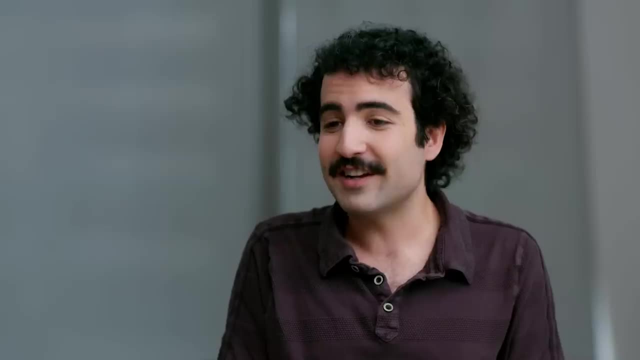 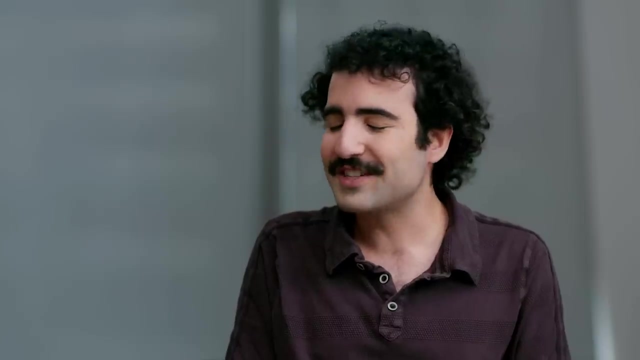 the night sky? Yeah, but if it's sufficiently far back, you're Right, and so we can learn a lot by looking at other galaxies and seeing what they were doing in their present. I suppose Just figuring out what's going to happen next is part of the issue. 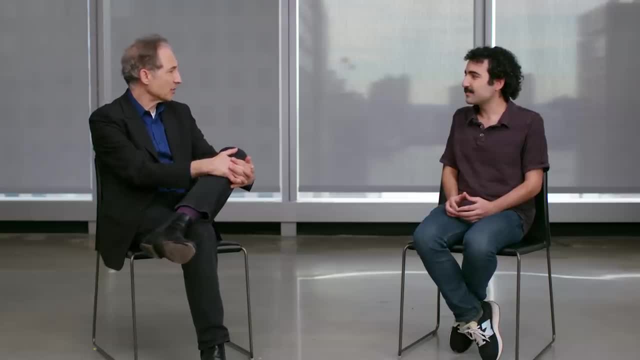 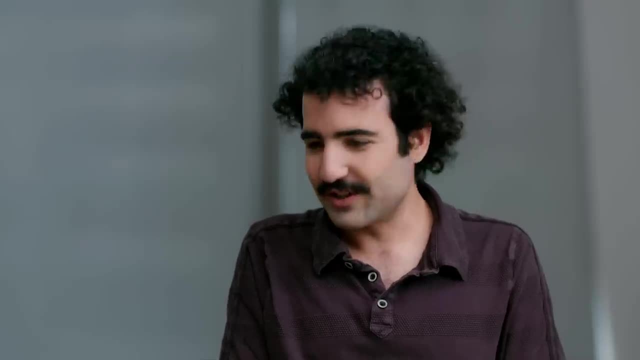 That's looking into the future, I suppose. And so have you taken general relativity, or are you taking that now? or I took a course on general relativity, yeah, But you learned about black holes and, Sure, One of the weird things and wonderful things about wormholes is that They are tunnels, if you will shortcuts from one point in space to another point in space. But once you have a shortcut from here to there, the beautiful thing is if you move the openings, time will elapse differently at the different openings. 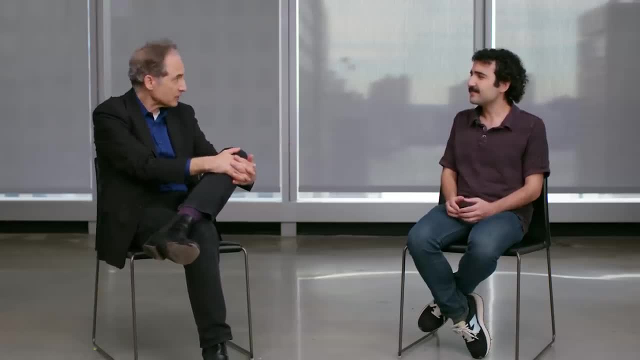 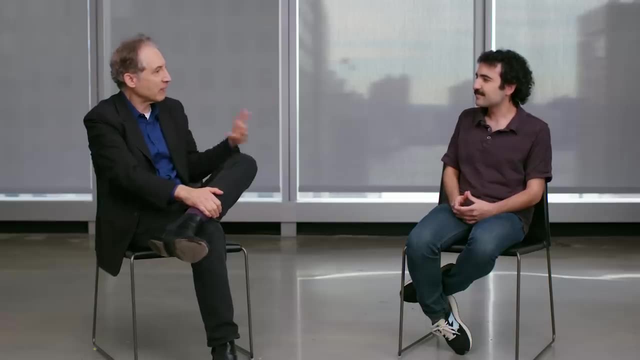 So there's a possibility of wormholes as time machines. Go one direction, you're going into the future. Go the other direction, you'd be going into the past. But that of course raises philosophical and logical Paradoxes. 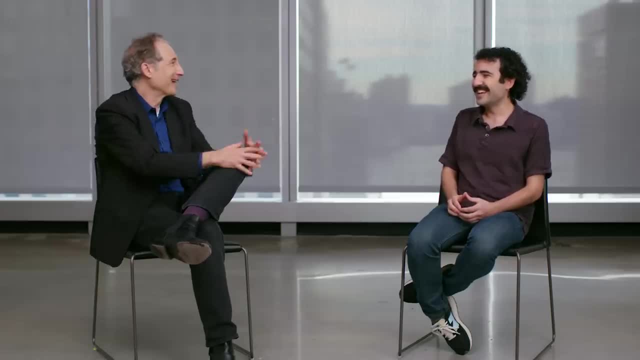 Paradoxes of some sort. So what do you think? What do you? I throw it to you. Yeah, I've heard a few different theories that people posit, like maybe it is back to the future and you really change your own universe. 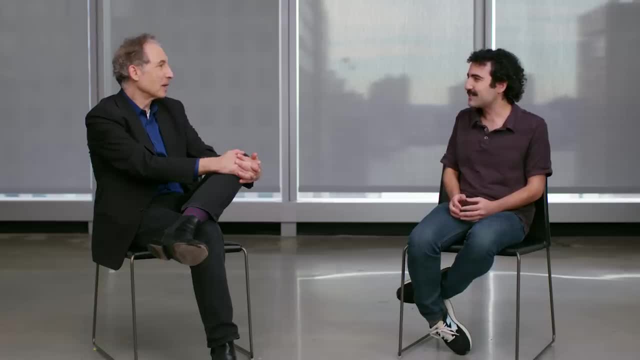 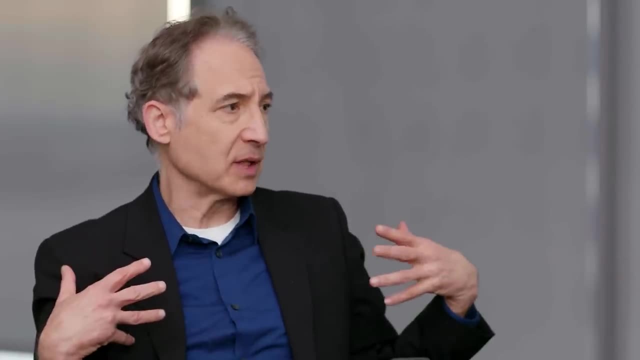 I've also heard people say that you could have multiple universes spawn from this event, or something along these lines. If you're going to be able to change the past, that's the one that resonates most with me. I think the same. Yeah, So you go into the past. You can prevent your parents from meeting, but you're preventing them from meeting in a parallel reality, which means that you will never be born in that reality. but the origin of your birth is still completely understood. 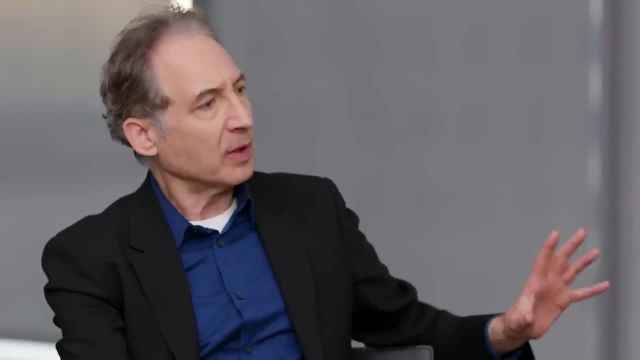 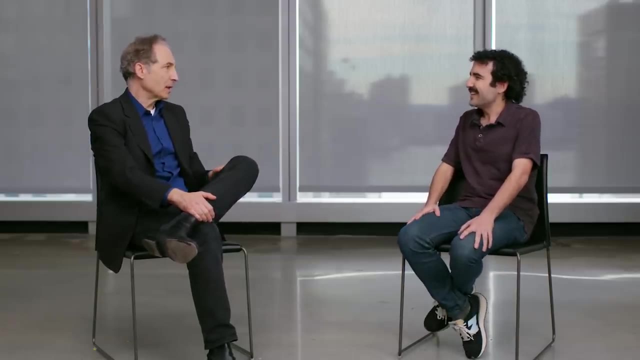 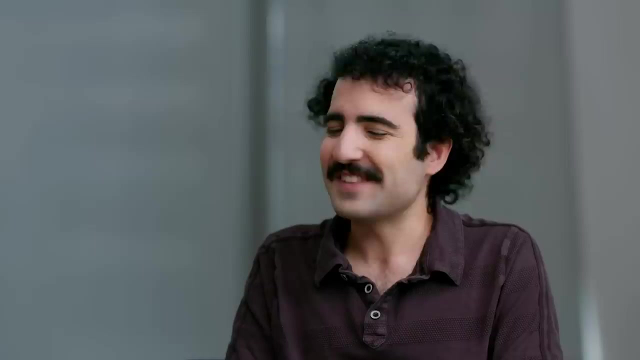 It was in the universe from which you originated. Another one that's more subtle is: the laws of physics may prevent you from interceding Right, And that raises uncomfortable issues for many people. Yeah, That's one of the things that's having to do with like free will. 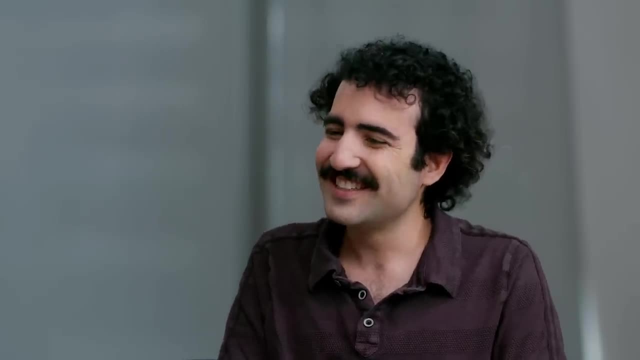 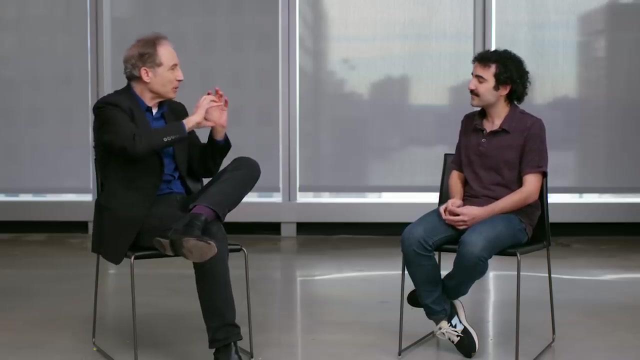 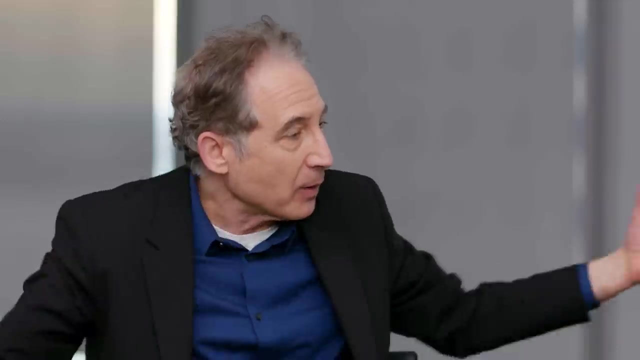 I'm immediately uncomfortable. Yeah, So that one. there's actually some people like Joe Polchinski, who did some wonderful studies of billiard ball tables, where you imagine a billiard ball goes into a wormhole, comes out and hits the very ball that was going into the hole and in that way, if it. 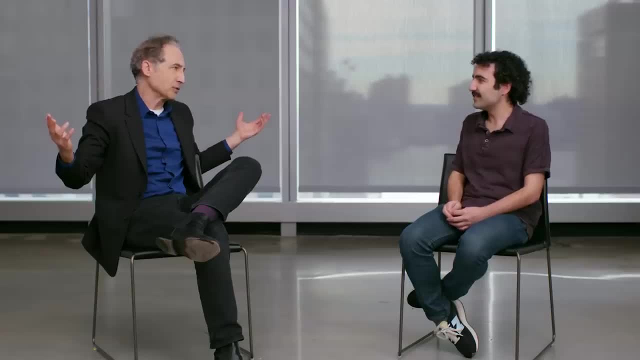 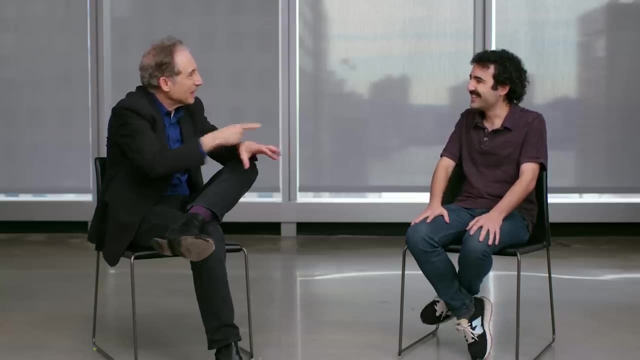 could knock it off. course, we seem to be in some logical paradox, Absolutely. But the finding was the ball can come out and just sort of graze The other one, but it can't affect it enough to prevent the sequence of events from happening. 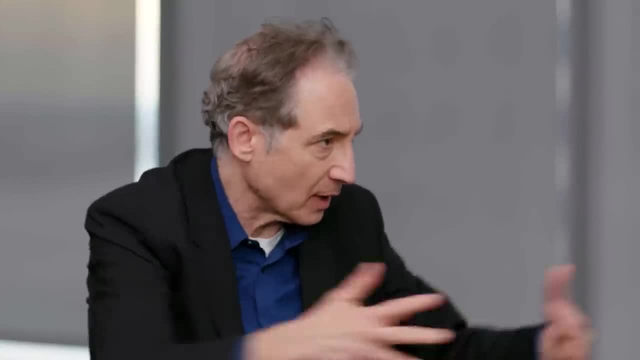 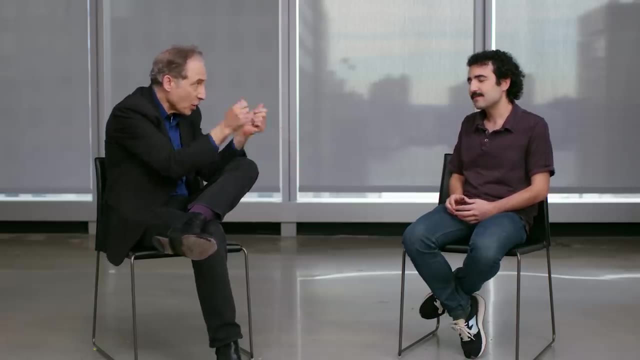 And the way I like to think about it frankly is if there's one universe, not parallel universes like in the other solution moments in time just are, They don't change. The whole point of time is the variable along which change can happen. 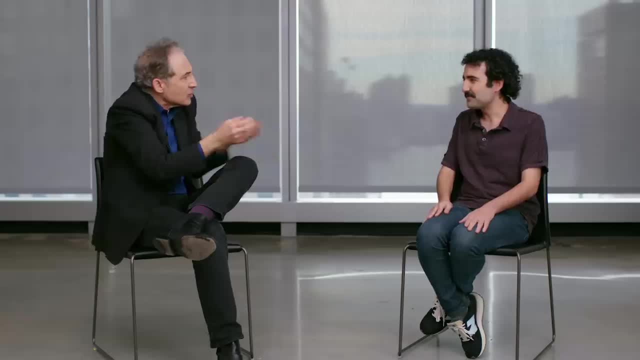 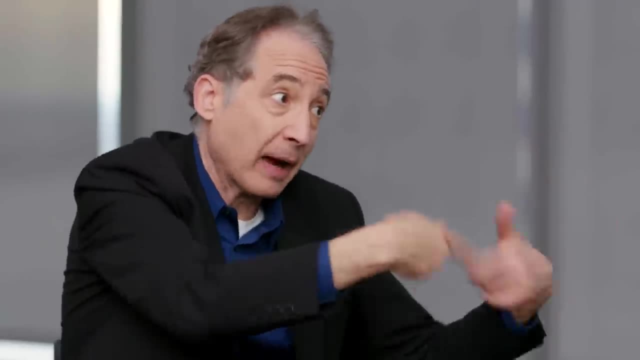 So if you have the atoms of time, the individual events, there's no conception of them changing. Yeah, If there's no conception of influences were in play that allowed your parents to meet, they will always be in play because you were always part of that moment. 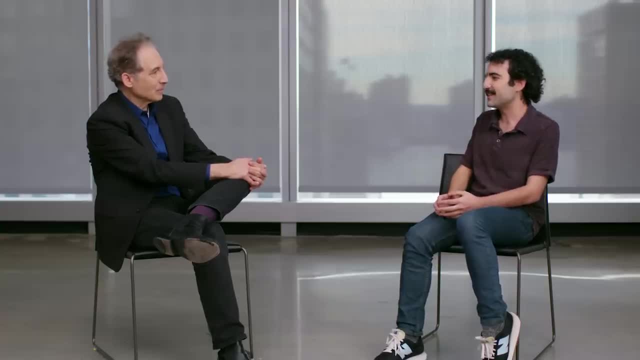 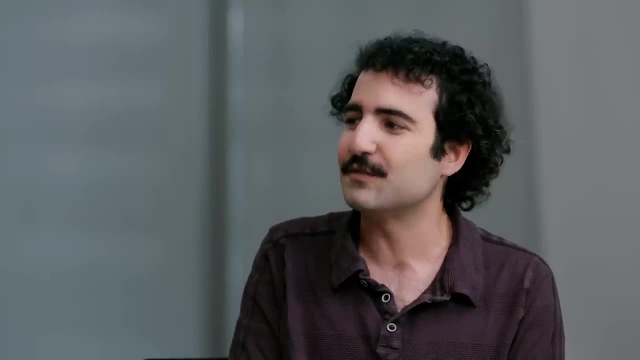 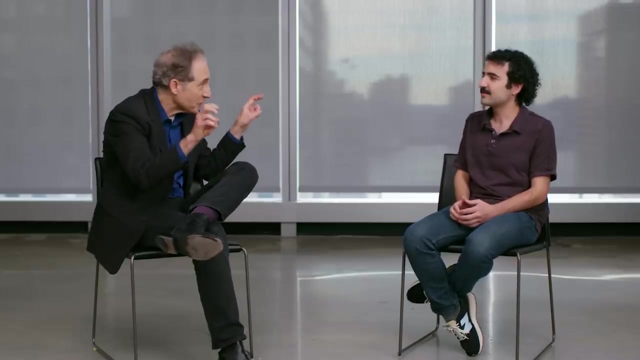 Do you think travel back to the past is impossible because of a deep physical, mathematical reasoning or just because of all of these problems that you've been talking about? I suspect that when we fully understand the mathematics of the final physical laws, if we ever come upon them, I think there's going to be something built up. 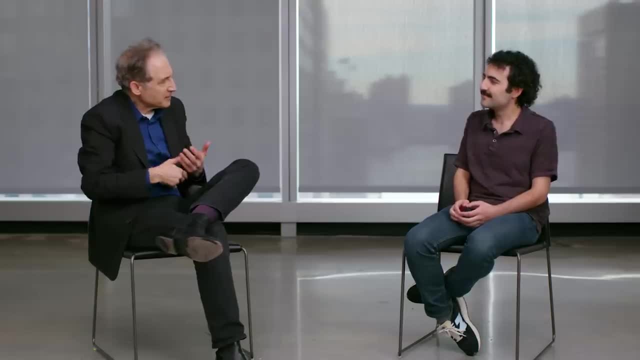 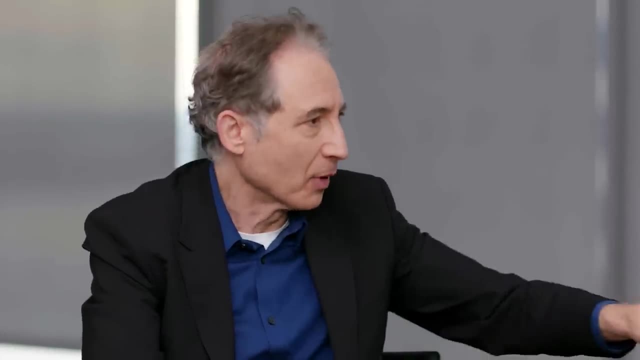 I think there's going to be something built up. I think there's going to be something built in that prevents this kind of free travel to the past. But sometimes I wonder if that's just coming from a more emotional place where I sort of want the world to be safe from these kind of paradoxes. 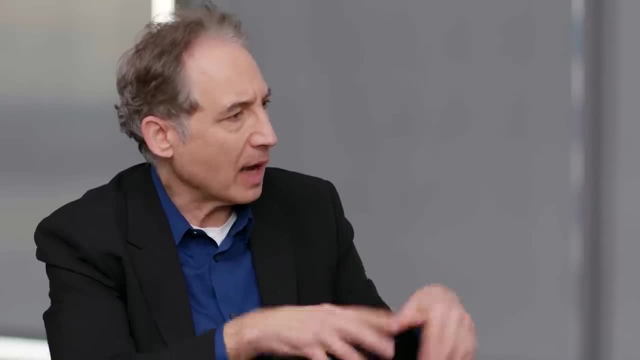 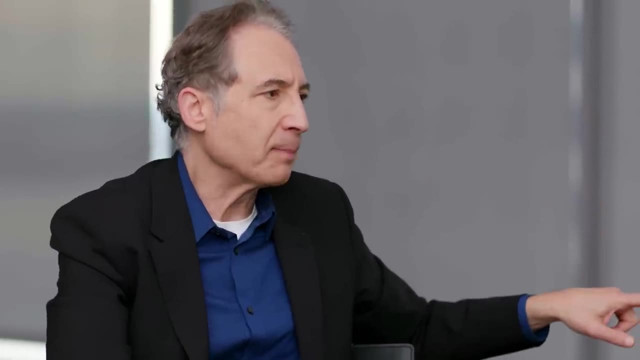 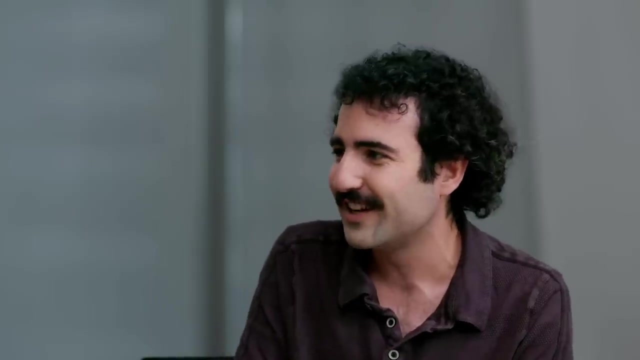 So what's pretty clear, based on any of the hypothetical proposals for traveling to the past that have come out of physics, you can't travel to a moment in the past before the first time travel machine is built. Sure, You know the twin paradox where you fly off, looks like you're moving fast, but to you 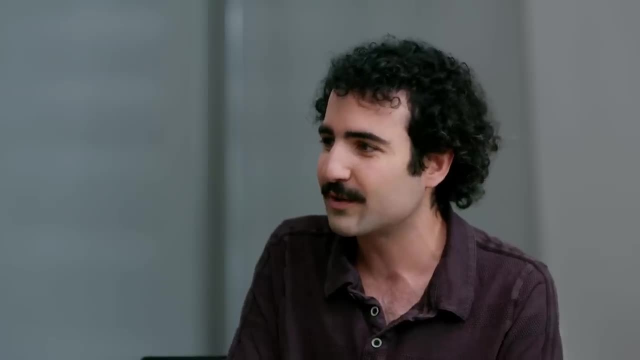 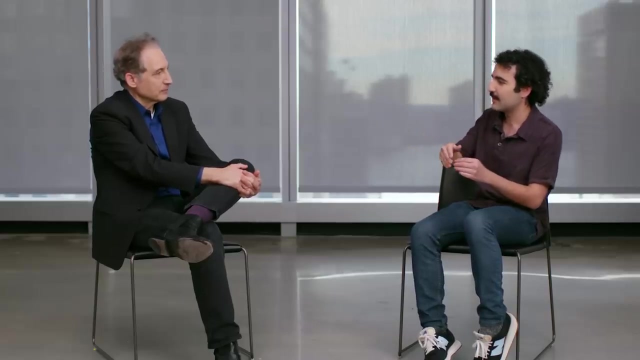 it looks like the other guy is moving fast. so who actually ages more? who ages less? A resolution I've heard is that because you have to be going away and then coming back, you had to accelerate at some point, and this breaks the ambiguity. 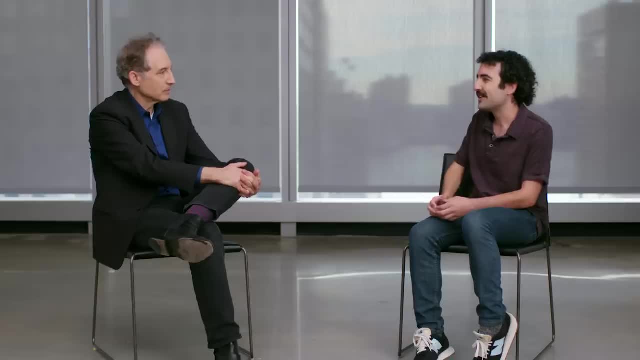 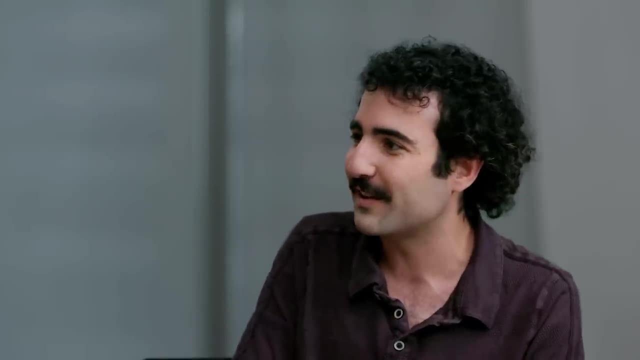 What if, say, the universe isn't flat? What if the universe is curved and you go off in one direction and then you come back in the same direction. you pass by the Earth. who's older then? Yeah, Do we have an answer? 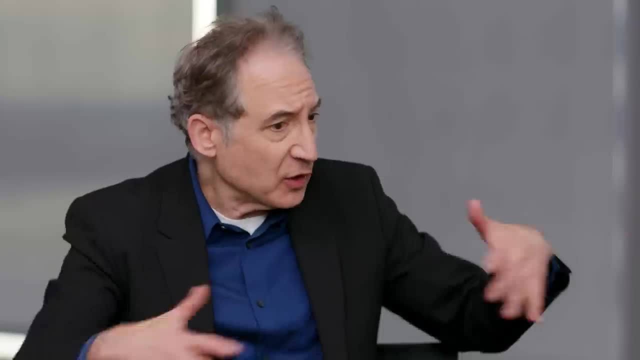 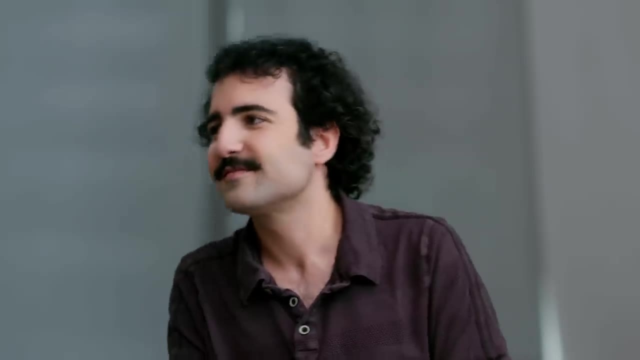 Yeah, we do have an answer. So the simplest version of that is: imagine that the universe has the shape of a donut. Imagine I'm on the circular part of this donut universe and imagine I turn on two laser beams sending a beam of light going to my right and to my left, and these beams will 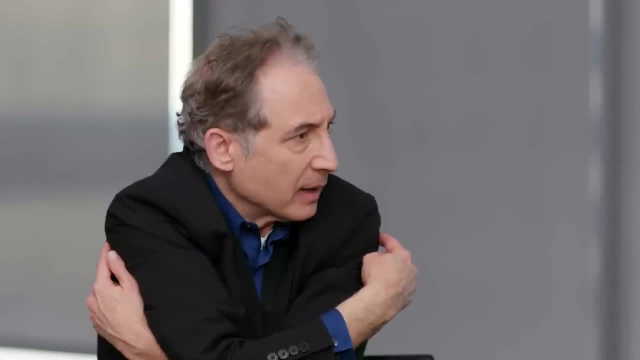 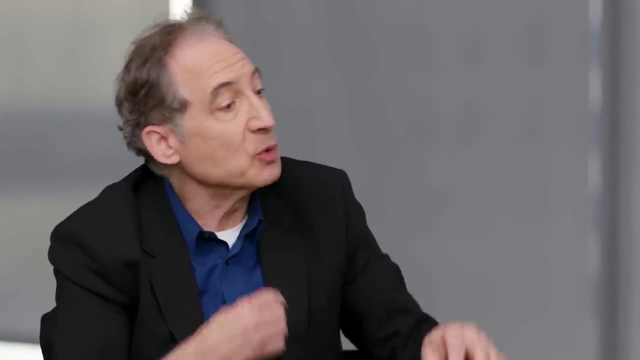 go around the entirety of space and they'll both come back and at some point they will hit me. Imagine they hit me at the same moment From my perspective. Now imagine someone's moving relative to my frame of reference, say to my left. 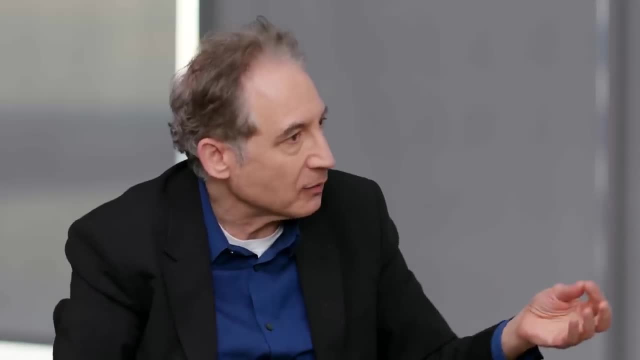 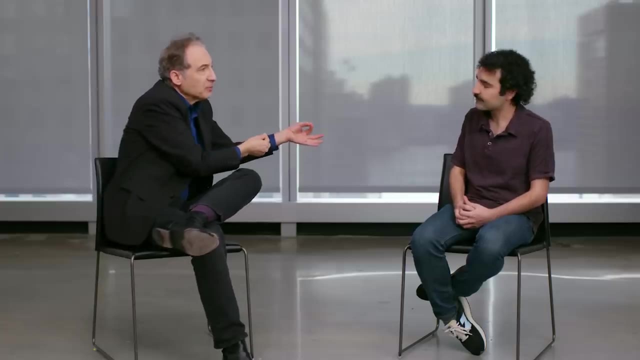 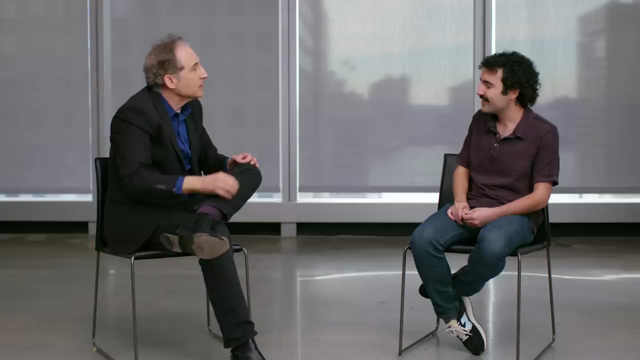 They do the same experiment. They fire the beam of light left and right, Notice that the beam that they fired to their left will have to travel farther to reach them because they're moving away from it, whereas the beam that they fired to their right will not have to travel as far because in some sense, they're moving toward it. 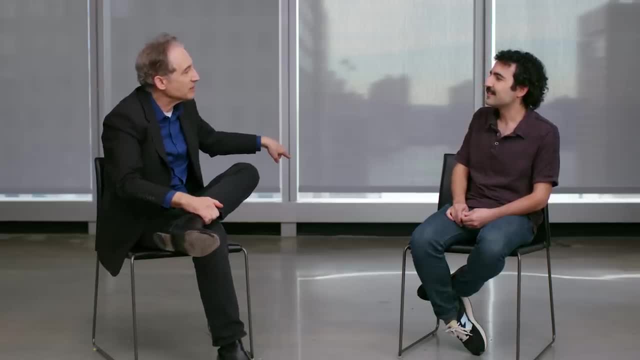 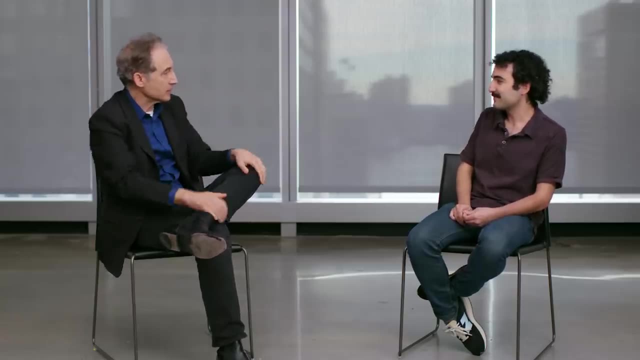 The two beams of light will not hit that moving observer at the same moment. To you, To them, To them, Wow. Which means that there's a preferred frame of reference in this universe. Everybody is not on equal footing as they are when we teach to freshmen the special. 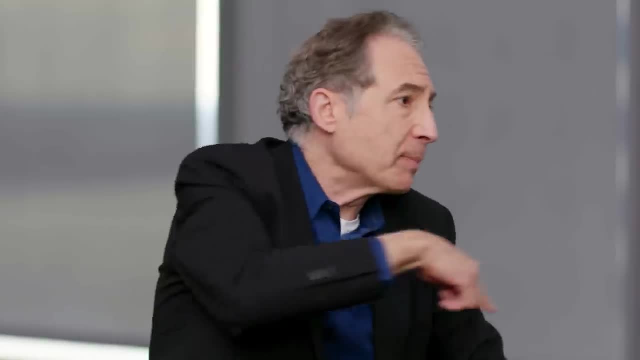 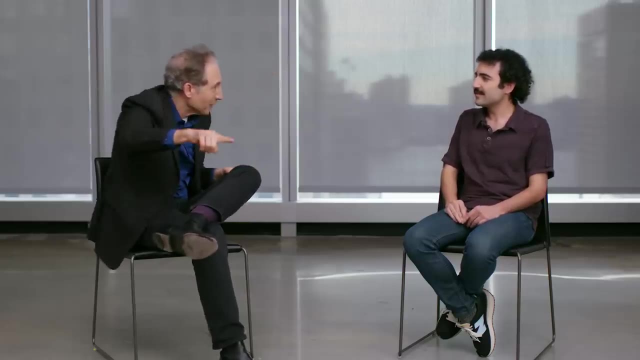 theory of relativity. That's right. Exactly Me, for example. No, Everybody else is moving relative to me and it's real motion. So everybody else will be like the moving twin: They will be younger and I will be older. 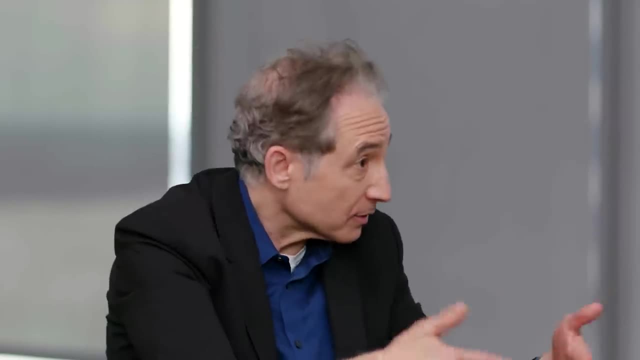 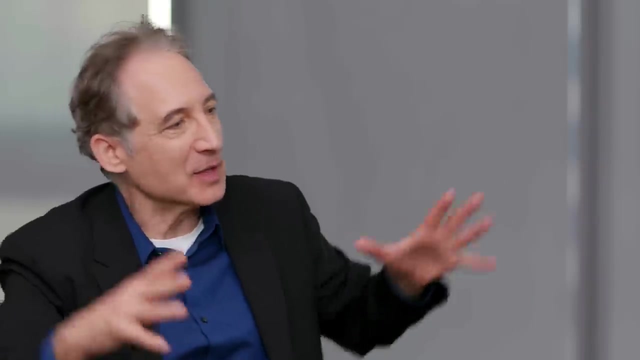 When you think about past and future on a cosmological scale, There was a long period when there were no human beings in the universe. The fact of the matter is, there will be these two long stretches, with our presence being sort of a flicker in between. 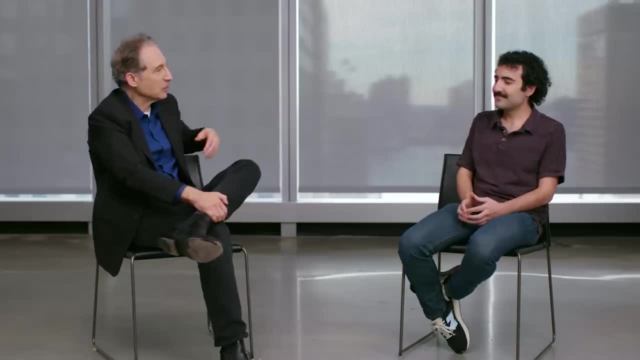 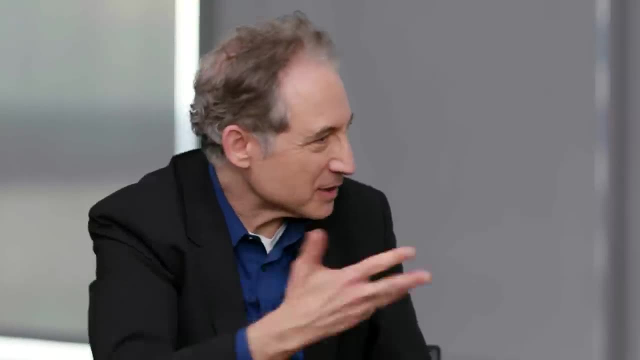 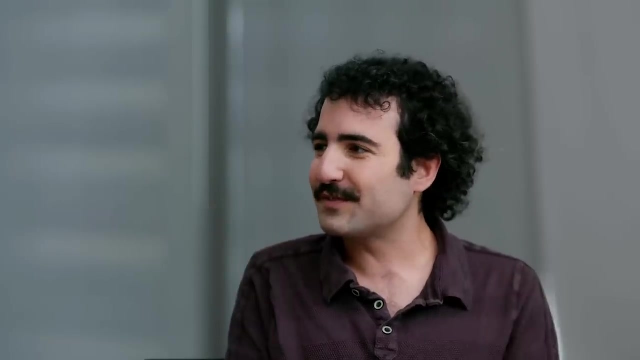 Does that thought inform anything about how you live in your brief flicker, within that brief flicker? I rage against thinking like that. Too defeatist, Too defeatist, I think that's the perfect way to put it. Yeah, It might be a brief flicker on a single mote of dust, like floating in a cosmic eternity. 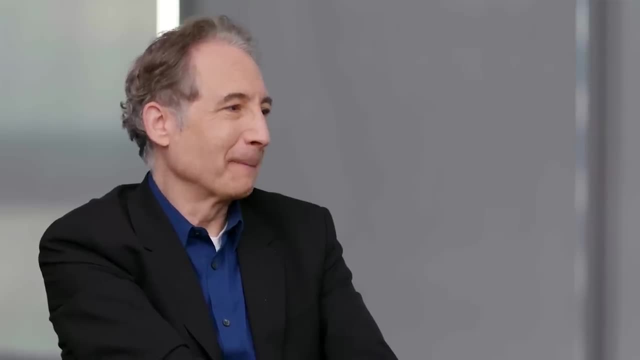 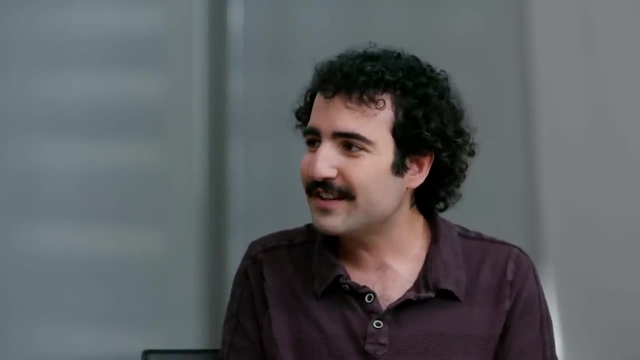 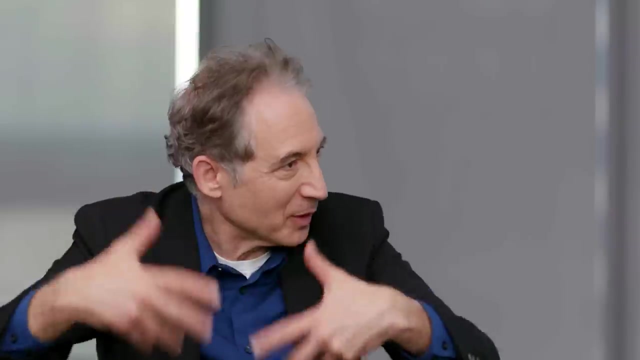 But it's everything. There's nothing else that I'll ever experience, And so, in a way, there's nothing else to me. There's an eternity, but I'm never going to see it, I'm never going to feel it. It can be debilitating to imagine an eternal future of sort of nothing, where none of what. 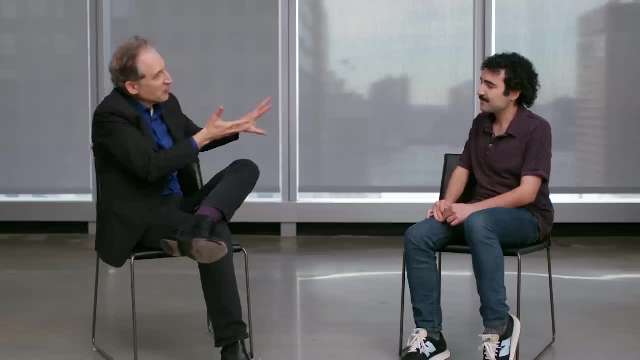 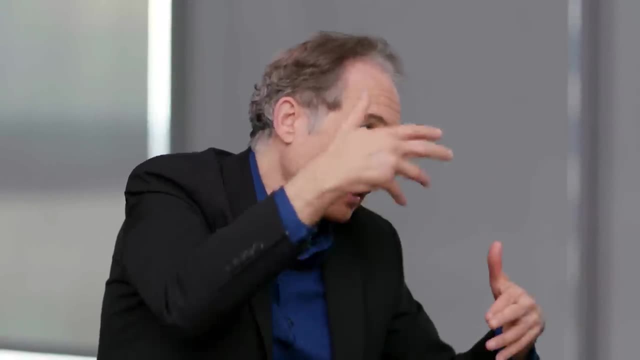 we do sort of persists. On the other hand, if you flip your perspective around and say: how remarkable is it that we have this brief moment that allows us to think and feel and love and explore and illuminate, Wow, how wonderful is that. 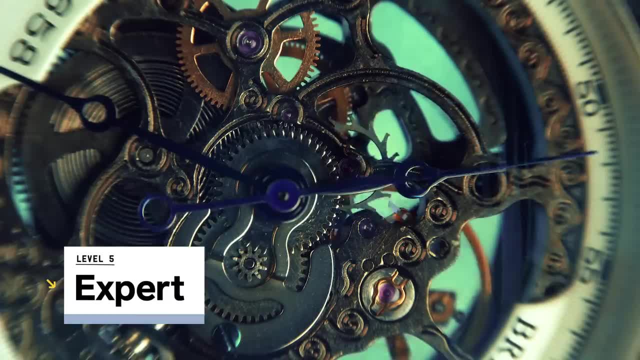 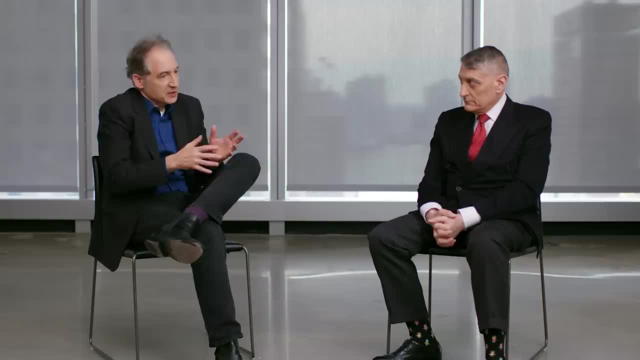 Yeah, So often, when we try to give the basic idea of what time is, I'm fond of saying: look, space is the language that allows us to say where events take place, And time is the language that allows us to Yeah. 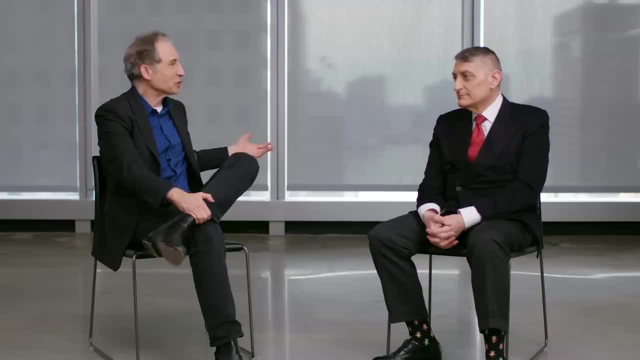 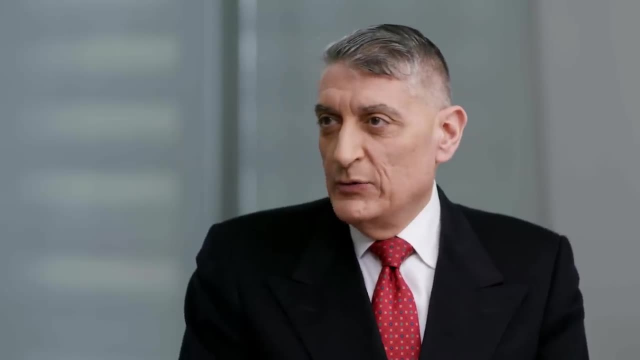 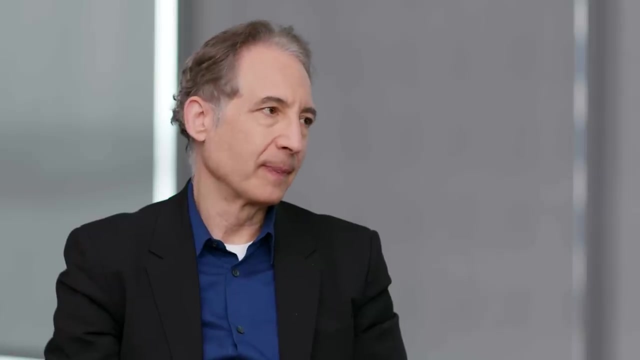 us to specify when they take place. Where would you jump off from there in trying to give a deeper understanding of the basics of time? Maybe part of the distinction in between time and space it's that you have a clear, irreversible evolution. So how to explain what time is? 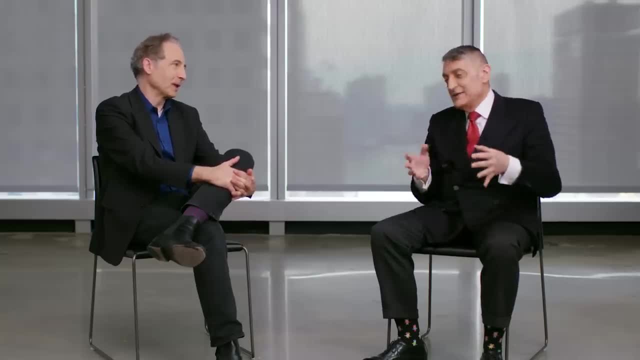 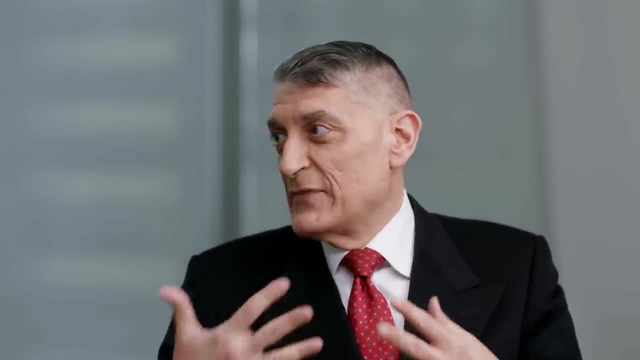 Well, it's a parameter that is measured by clocks. I mean, at the end, this is what we know And allows us to talk about change, And also that we know how to describe in terms of some set of equations, Which gives a clear sense of causality. 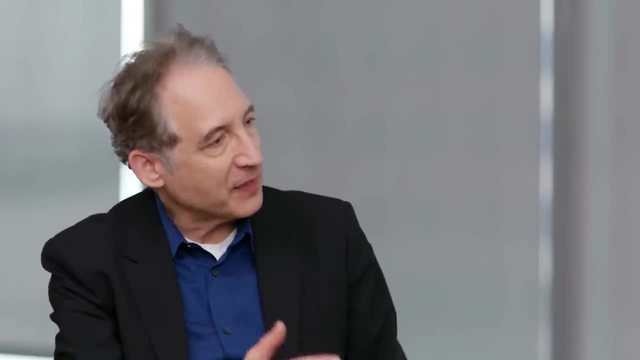 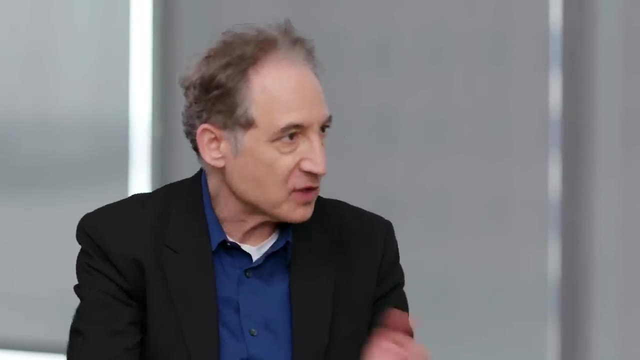 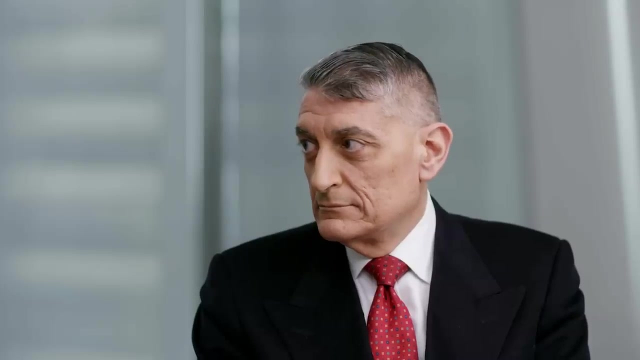 To note our recent paper where we were thinking about Einstein's ideas of special relativity, but in a setting where the global shape of the space-time we imagine there might be a curled up dimension of space, a circular dimension, and thought about how special relativity 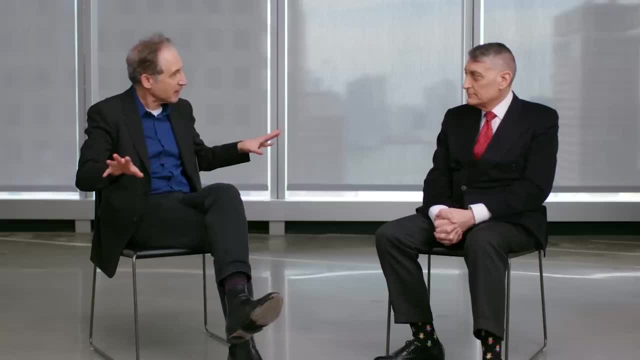 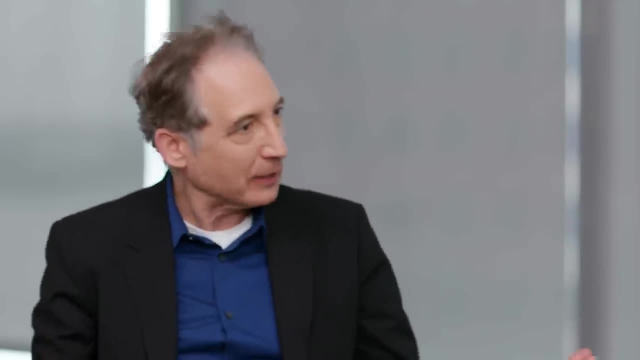 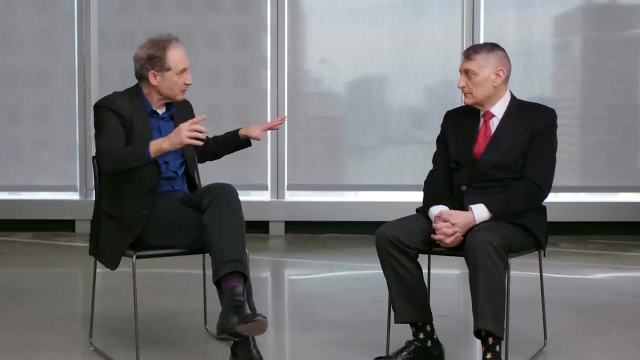 works. in that setting We came to a result. in this very basic setting You can send signals into the past, not in a way that will violate causality. Did that surprise you? That by going from the usual topology that doesn't have a closed part of space, but making 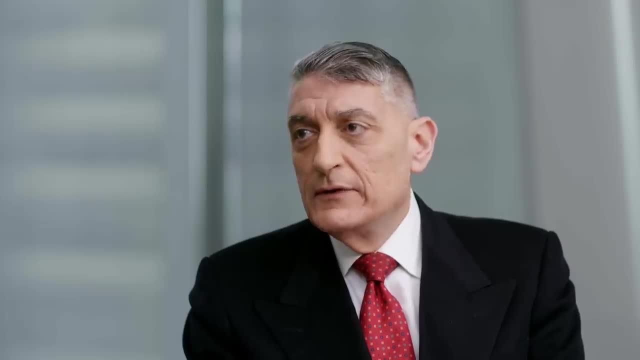 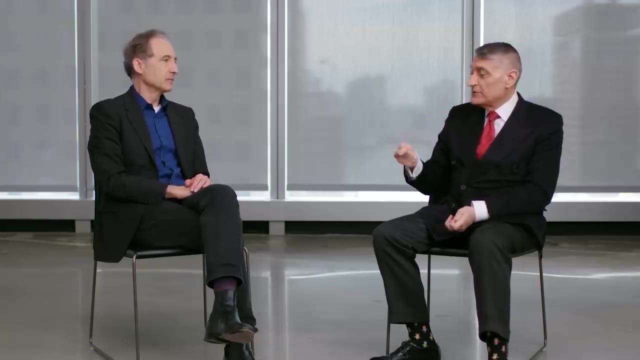 that one change you can have this radical impact. I found quite surprising that you could have this exotic behavior of signal propagation in a system that was extremely simple, totally classical. There was nothing weird, Exactly Except one dimension that was compactified was identified on a circle. 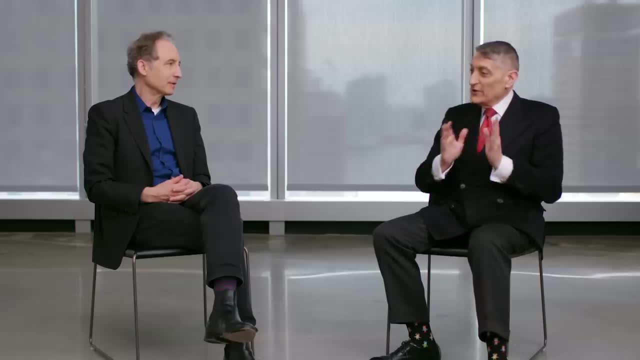 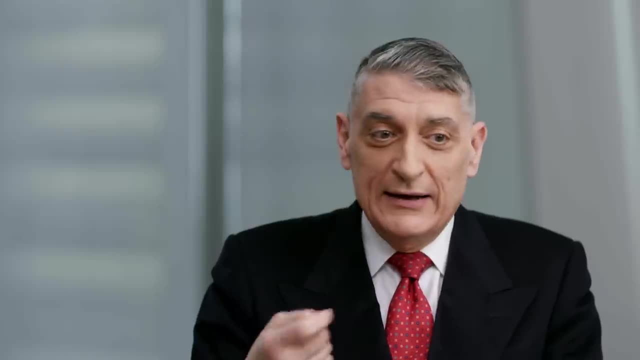 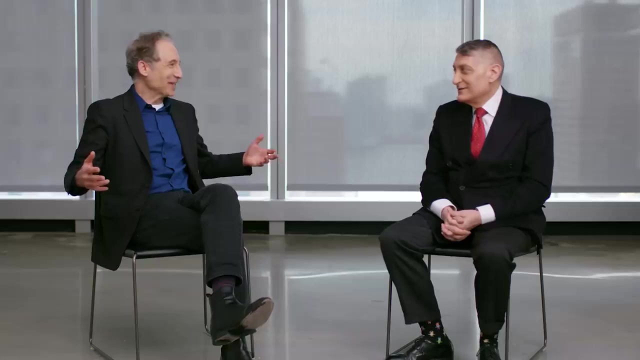 Actually, even the standard vanilla causal structure of special relativity may give some very unexpected behaviors when you combine it with other simple modifications of just the flat space-time. And the beauty of it is it's not like there is some high-powered mathematical methodology. 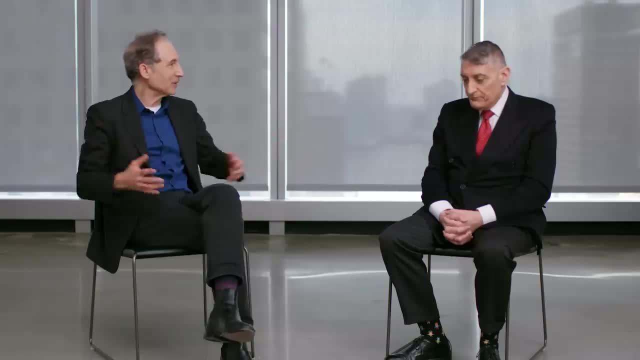 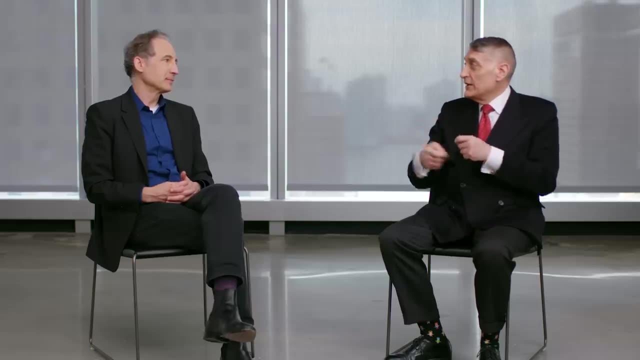 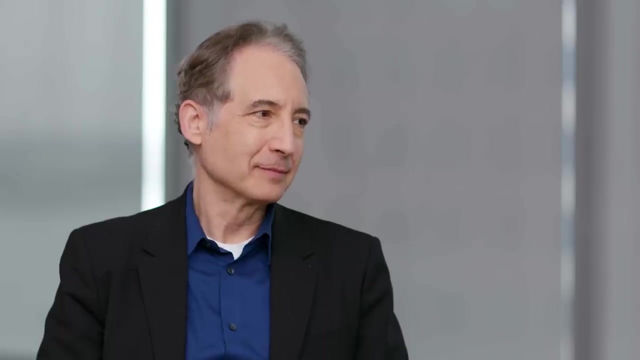 Straightforward algebra that a high school kid knows. Yeah, A high school kid would know- is all that you need to extract these unusual results. And they were unusual because, even if you do not violate causality, we discovered that a fast-moving observer that could be us on a rocket could send signals very far and 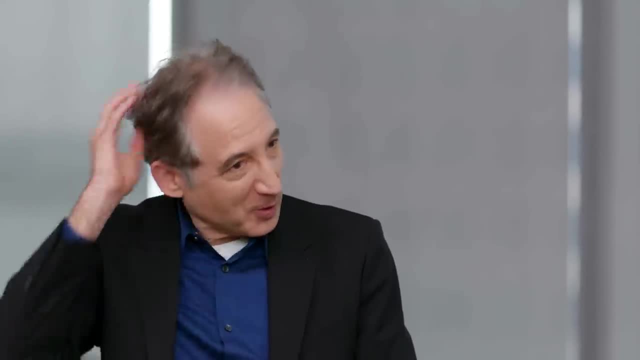 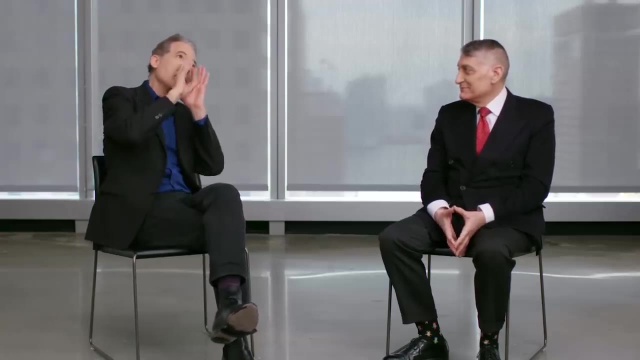 then back in a very small time, And so the old idea that of course we always hear about that if we ever make contact with extraterrestrial life, they're far away. we can't really have a conversation because we'll say hello. 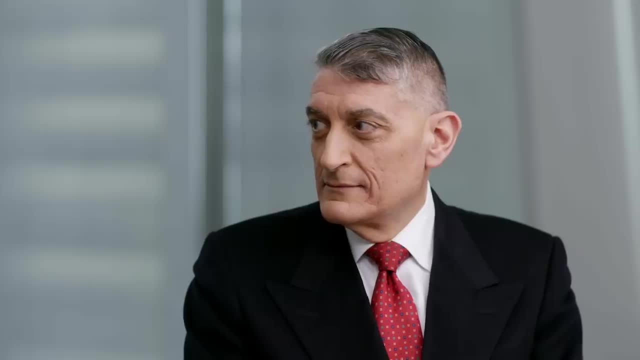 And then, like 10,000 years or 100,000 years, Yeah, 10,000 years later they'll answer us because they'll take that long for the signals. But at least in this setup, which we don't know is true of our universe. but if it were, 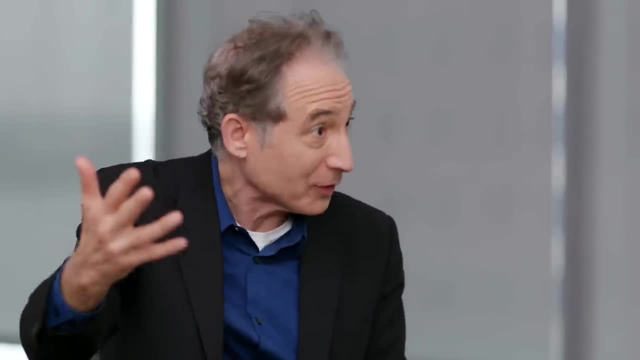 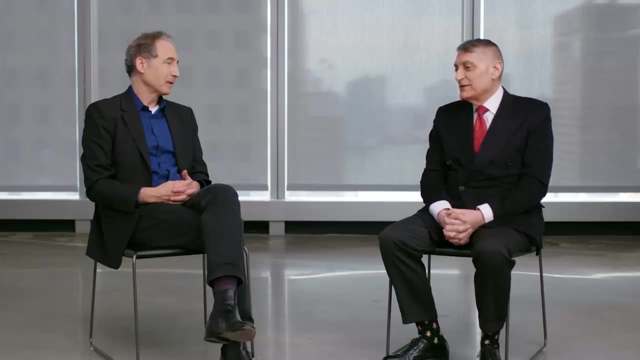 then you could have a real-time conversation over arbitrarily large distances, which is That was unexpected, Yeah, And so that shows how even ideas that seem to be well-settled and well-understood have surprises Like: why didn't Einstein realize this? 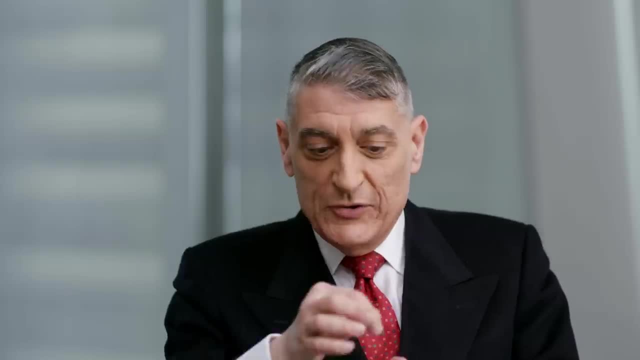 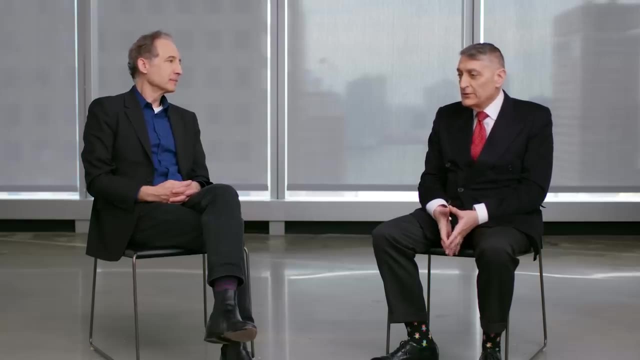 Yeah, Maybe the idea of living on a subspace, of being confined in this extra dimension, on a surface, may have been looked exotic, but definitely did not look exotic. after the 1990s, Many people have begun thinking about the possibility that space and time may be so-called. 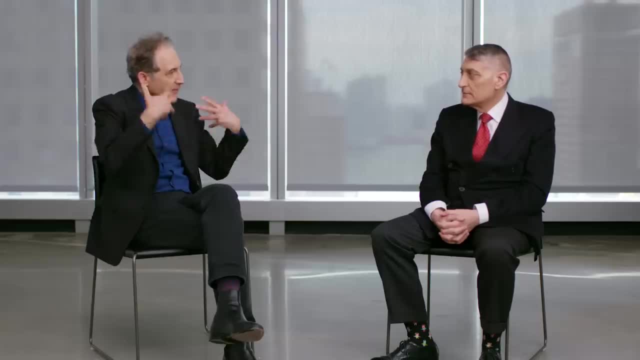 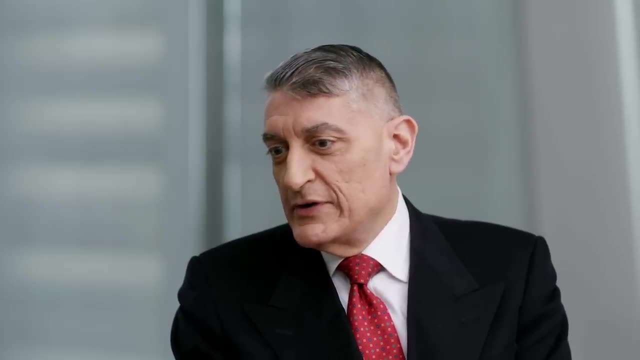 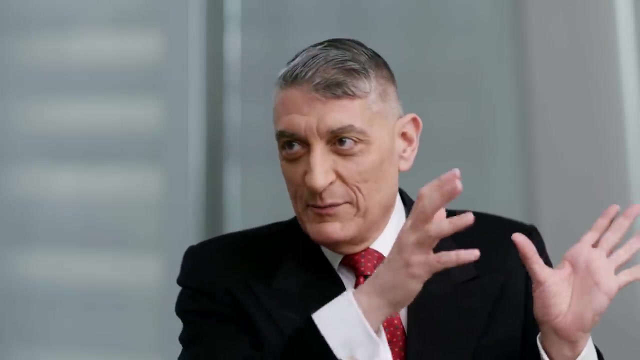 emergent quantities that they're not as fundamental as perhaps Newton or Einstein would have thought. Where do you stand on that idea? It seems not unthinkable. Saying that something is emergent will make full sense only when we have some concrete model in which space and time emerge and in which we make sense. 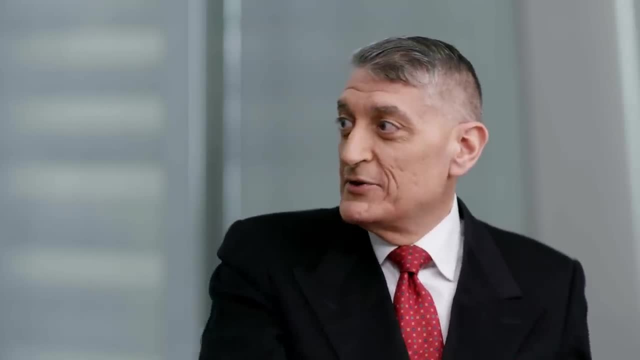 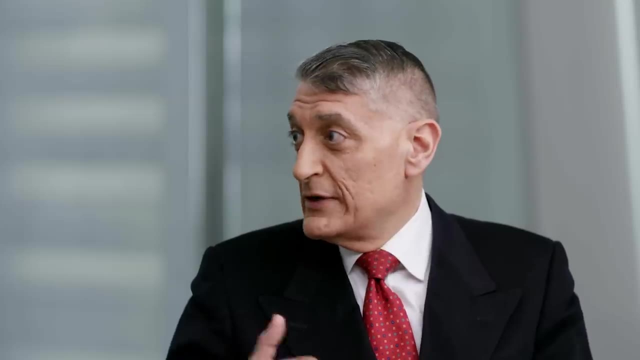 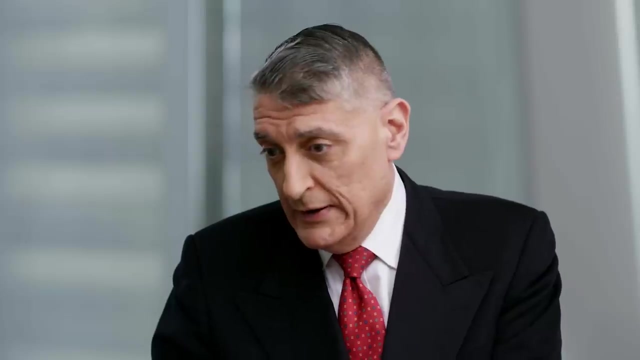 of this non-space, non-time description of a theory. I don't know if we are still at the stage in which I would say we begin to understand this scenario, because often I tell my students the greatest scientific revolution has been not in the 20th century. it has not been quantum mechanics, nor general relativity, nor special 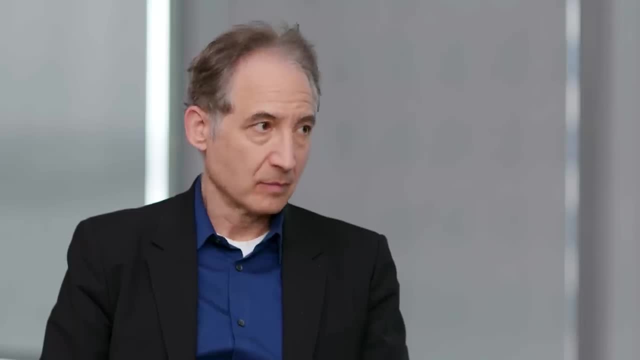 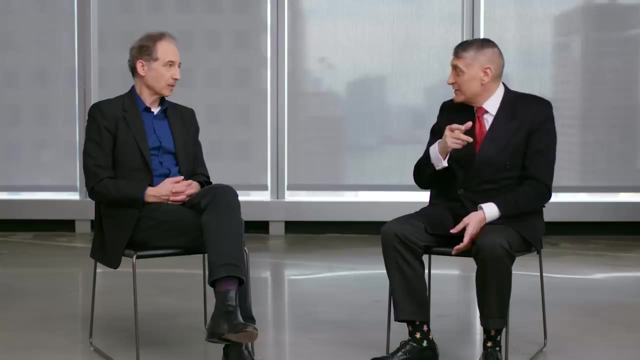 relativity. It has been a passage from the qualitative description of nature the quantitative one. When you pass from asking how to how much, then you understand something. And who do you credit with that? Is that Newton? Do you go Newton or a little bit below? 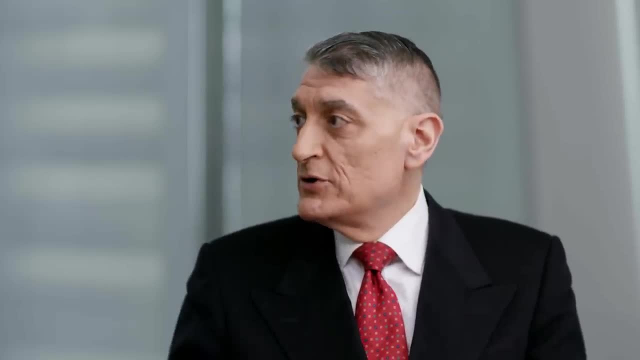 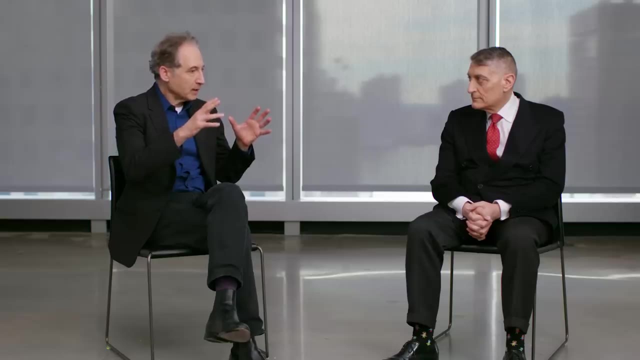 Do you go Galileo? I would say Galileo, Newton. Of course, the completion of this idea is Newton. One of the things that relativity also sheds a light on is what exists, that if someone's moving relative to me, what they consider now. 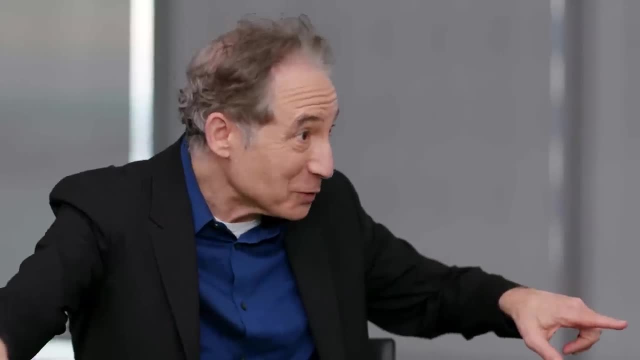 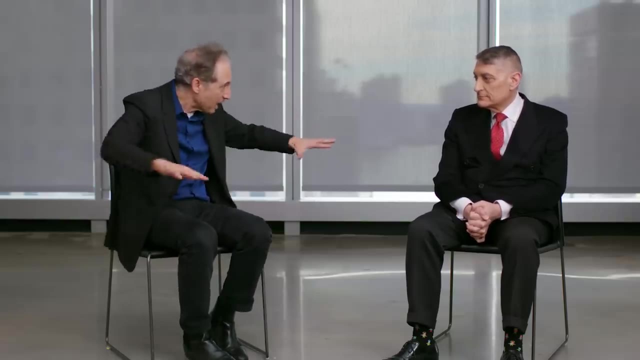 might be in my past. what they consider now might be in my future, which would suggest that all of time exists. much as we're willing to accept that all of space exists, Does that hold water? Actually, it resonates with me for various reasons. 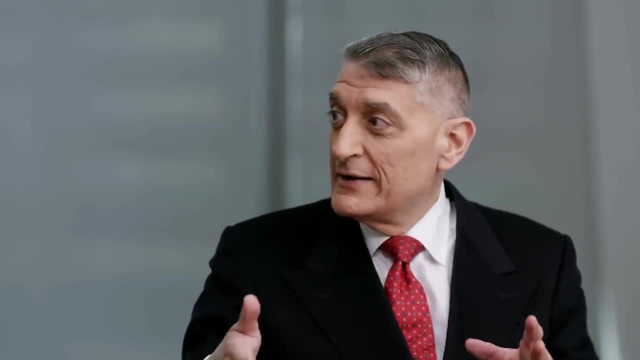 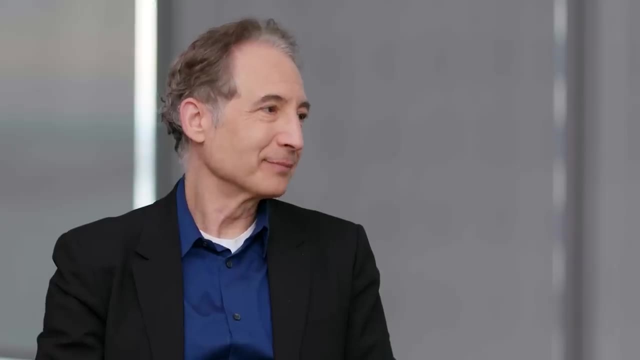 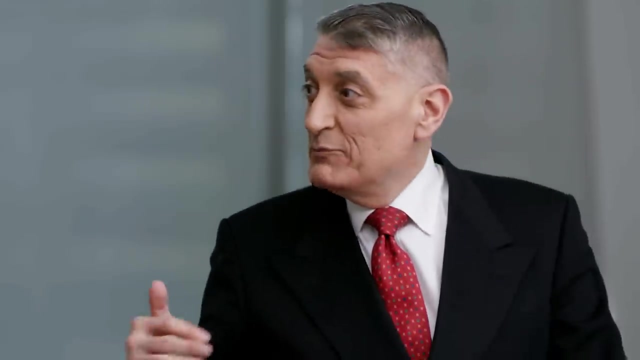 One is that, professionally, we use space-time diagrams, Penrose diagrams, a lot of diagrams where space and times are just two axes on a board. Yeah Yeah, In this article we have a line that goes up in time. By the way, this image also is the last image in Proust. 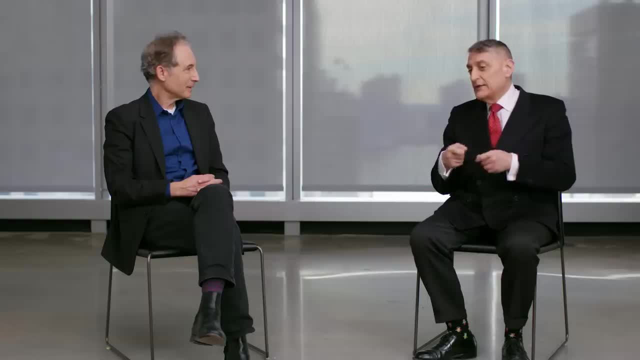 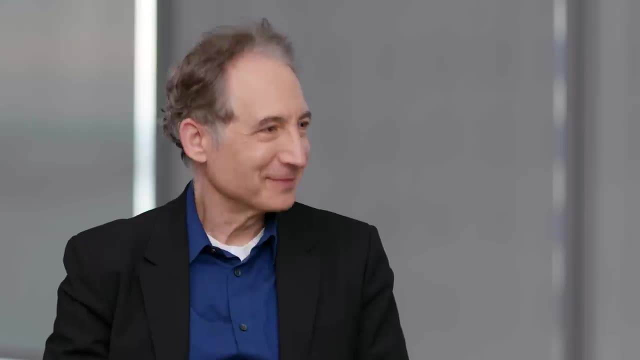 The last page, there is this beautiful sentence, which is also true, saying that if he has the time, he would like to describe people as being monstrous beings that extend in time much longer than in space. If it's equal to one, that's very true.